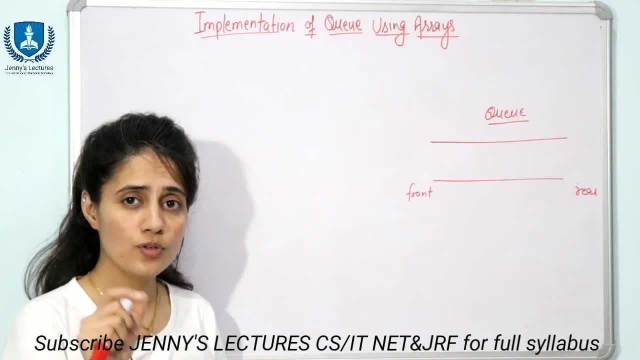 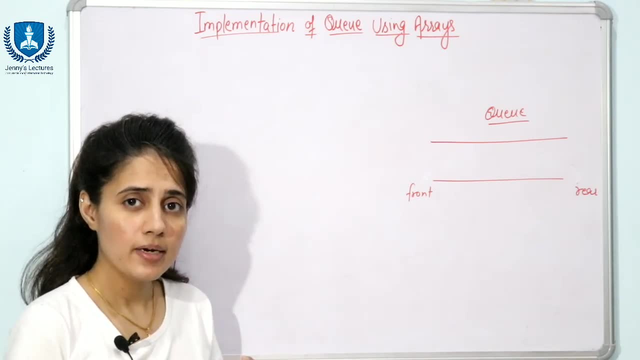 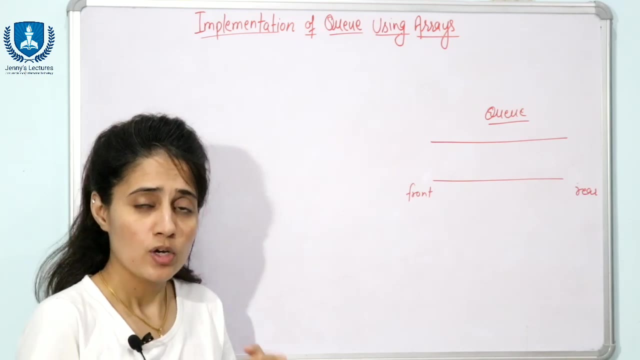 In the previous video we have discussed the introductory part of queue data structure right. In this video we will see how actually we can implement queue. Queue can be implemented either using arrays or linked list right, or using stack also we can implement queue. So in this video we will see basically how you can implement queue using arrays, right. So before 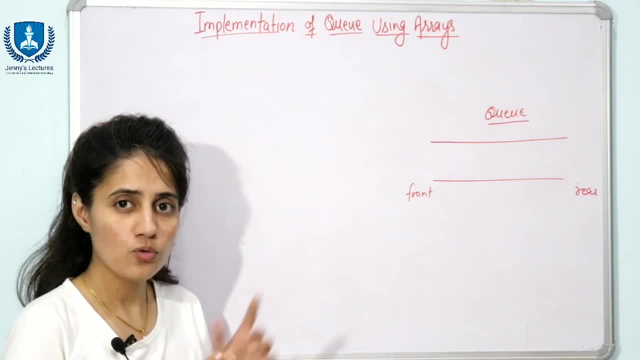 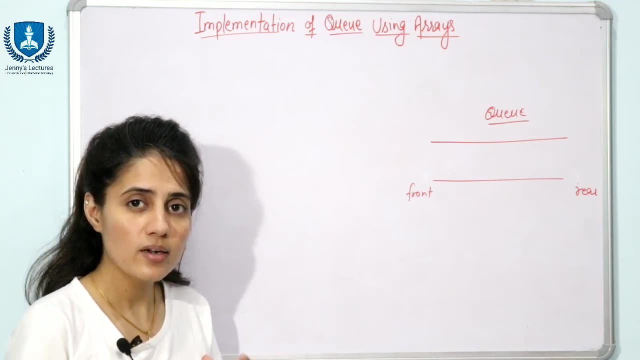 going to the implementation part, you must check out the previous video. you can check out in this. i button right What we have discussed. queue is a collection, or you can say it is a list, where the insertion is possible from one end and that end is known as rear and deletion is. 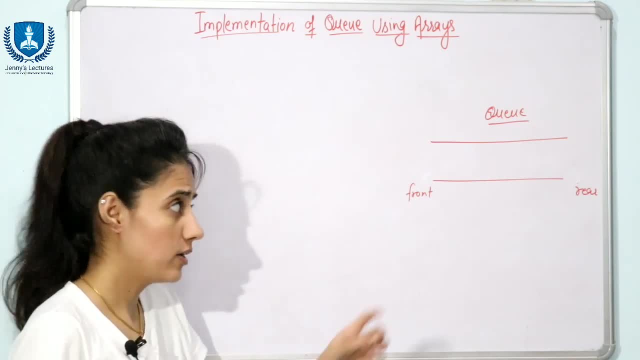 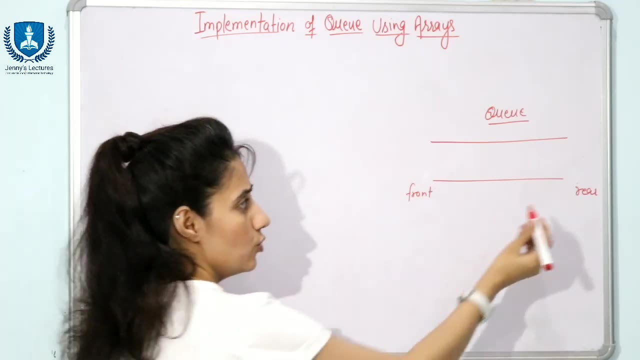 possible from other end, and that end is known as front. This is how logically you can represent a queue. This is what front, this is what rear right. You can insert data from rear end and if you want to delete the data, then you can delete from front right. 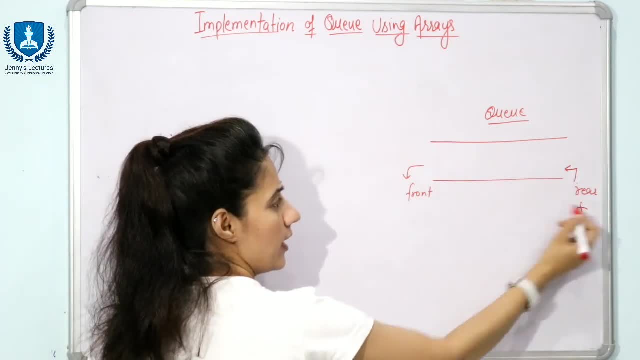 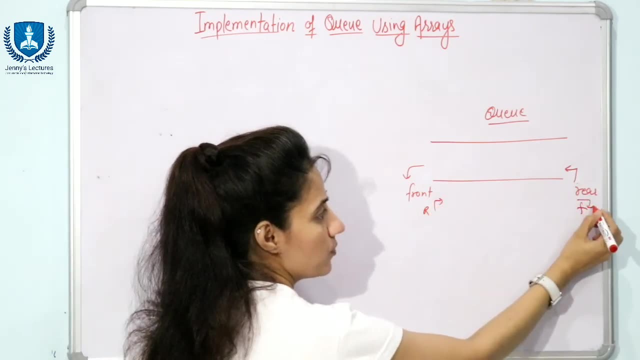 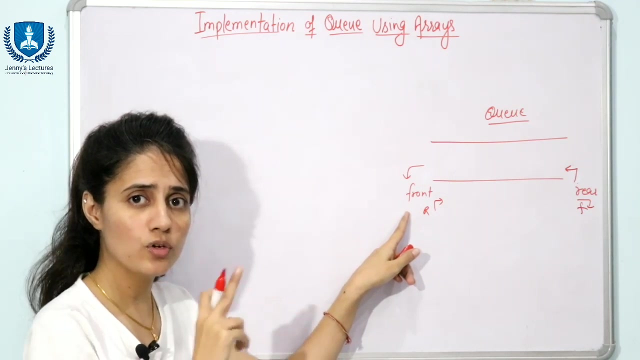 And if you suppose, consider here front and here rear, that is also fine. So insertion would be from rear and deletion would be from front right. You can choose any option, fine, but you have to take care of the rule of insertion and deletion. fine, Now how we are going to actually implement. 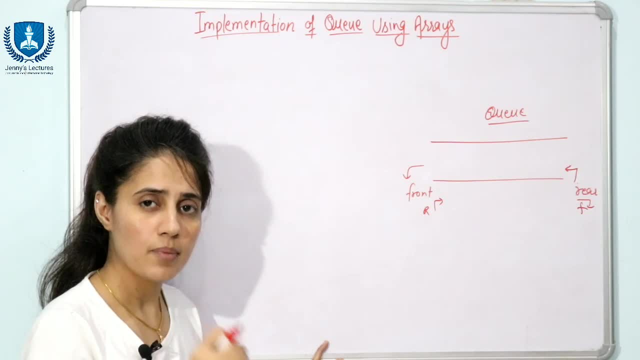 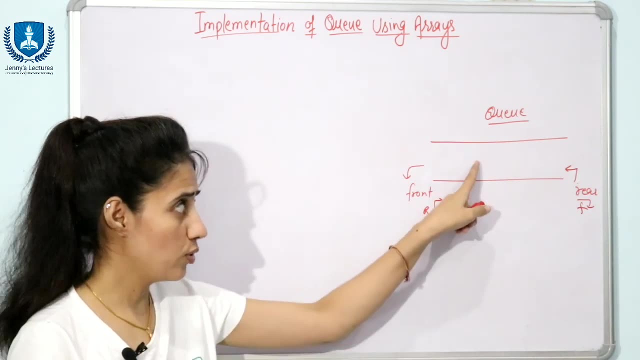 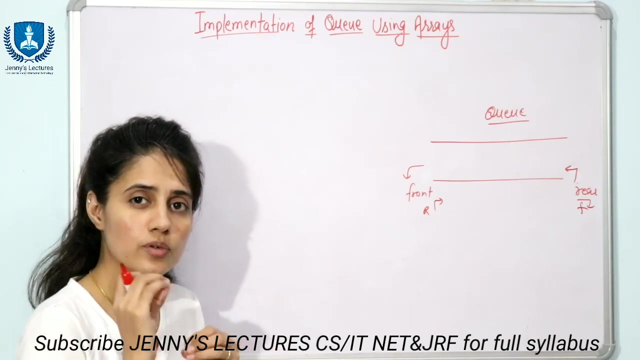 this queue using arrays. Arrays means we will use static memory location. First of all, obviously, we specify the size, how much data we can store in this queue right, The capacity of the queue and while implementation of the queue, you have to take care of that rule, that is, FIFO rule, because 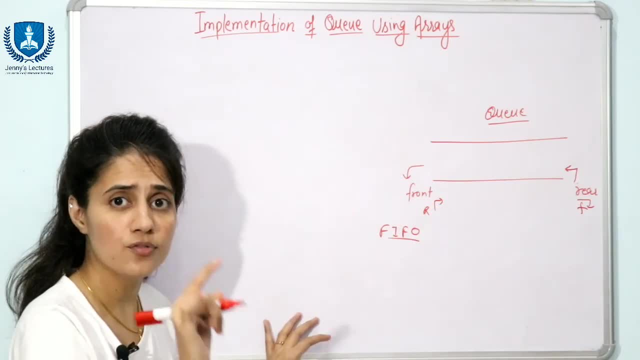 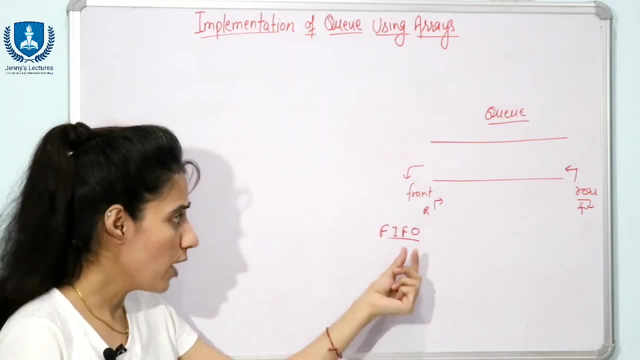 queue follows. what FIFO rule first in, first out? that we have discussed in the previous video, right? So obviously we are implementing this queue using array, so you have to enforce this rule here, and the time complexity for NQ and DQ operation must be the same, So you have to take care of. 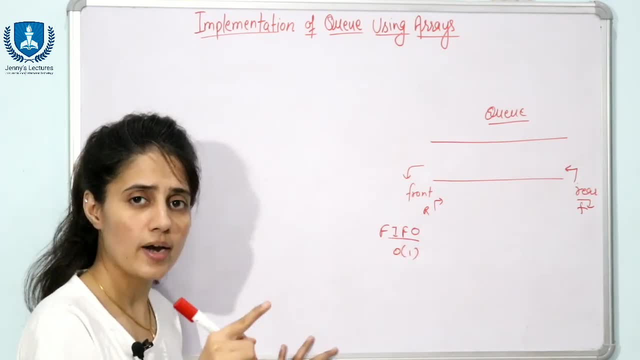 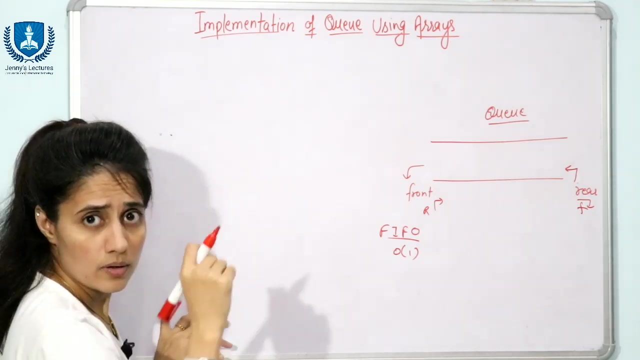 the order of 1.. See here: insertion is known as NQ and deletion is known as DQ, operation in queue: right, These are more technical terms in context of queue, So we will use NQ and DQ. Now we actually implement this queue using arrays. fine, Now how to define, how to declare array like this int array. 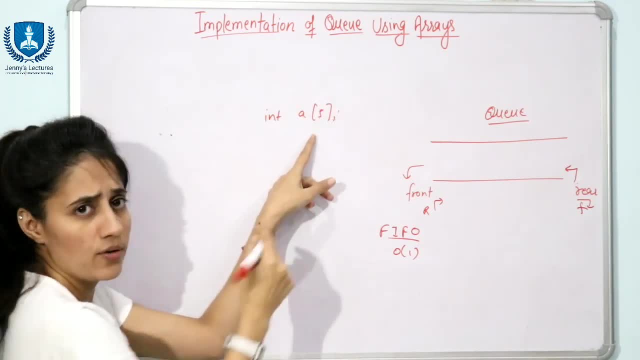 name and here size of the array, that is, any constant: 5, 10, as you wish, 50, 100, right? Here I am taking the name of the array and here I am taking the size of the array, and here I am taking the. 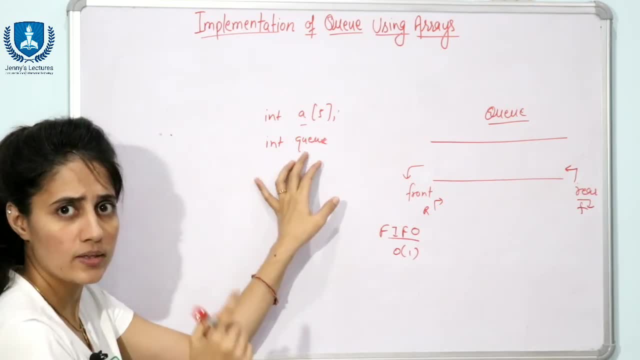 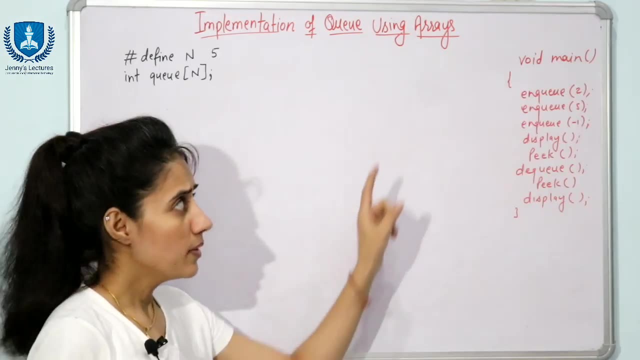 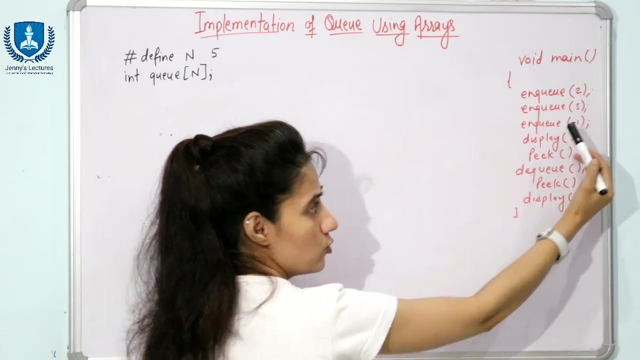 name queue, because I am implementing queue. that is why I am taking the array name queue and here obviously we will specify the size. Now, how to write down the code see. So now, suppose in main function I am calling first of all NQ function 3 times. I am passing this 2, here 5 and minus 1. 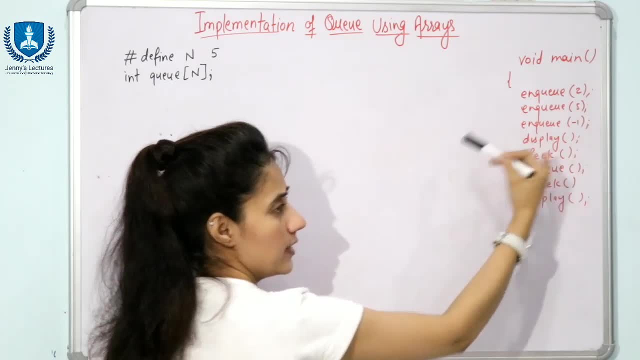 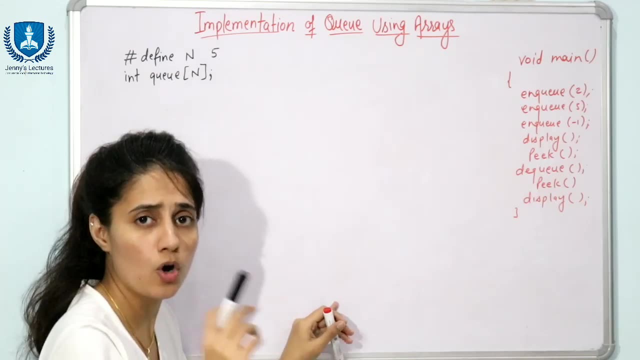 means first of all I want to insert 2, then 5 and then minus 1 right. After that we will display the content of the queue. after that, peak function, peak operation, fine. Peak operation means it is going to tell you whatever the front value of the queue, right. 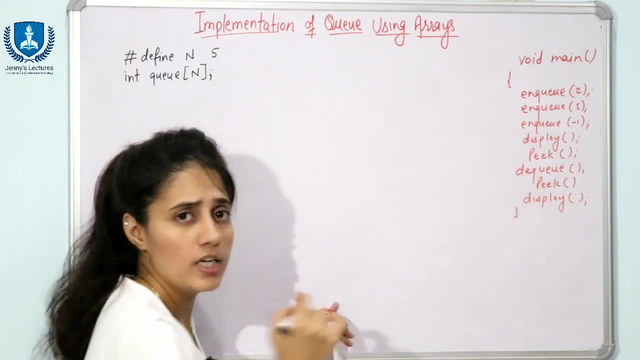 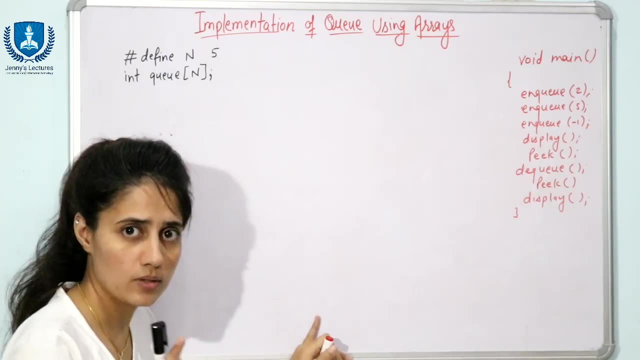 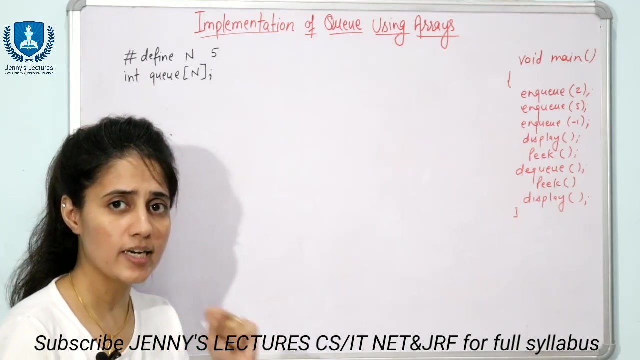 without removing that value from the queue Again, DQ function. DQ means it is going to delete the data from the front of the queue Again peak, and then we will display the content of the queue right Now. first of all, obviously we are going to declare the size we are, we are using what static 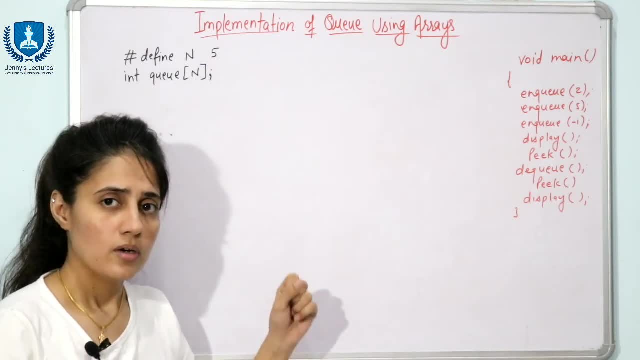 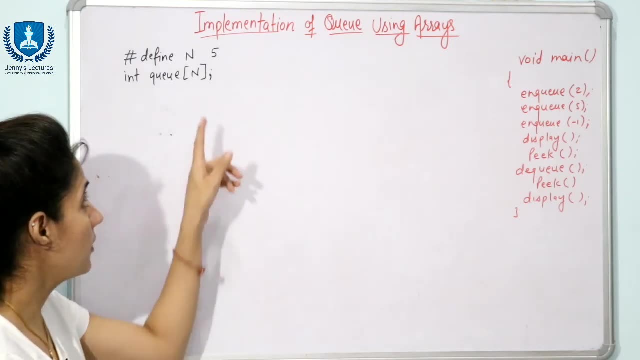 memory allocation here: fine. in array You can use dynamic array also, and for dynamic memory allocation you can use dynamic memory allocation. So we are going to use dynamic memory allocation. you can use linked list also fine, but here I am using static memory allocation. So I have defined. 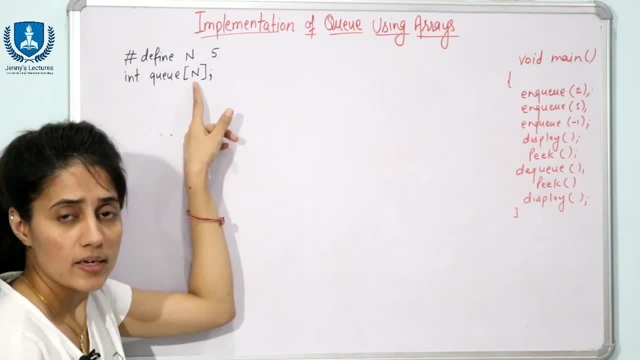 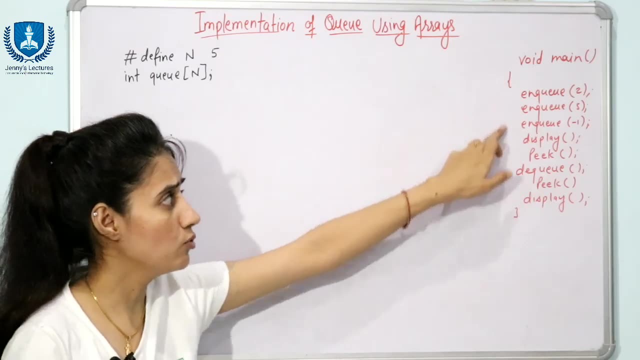 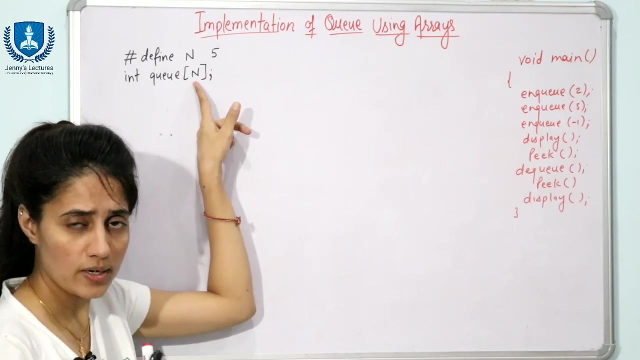 int. here the name is queue and size is N. See this queue we will use in all the functions. that is why I am declaring it globally, outside of main function and outside of all these function. after header file, directly right. and here I am not writing that size in constant term, I am using what macro. 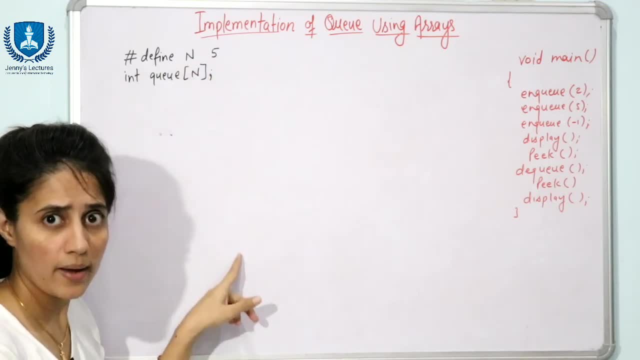 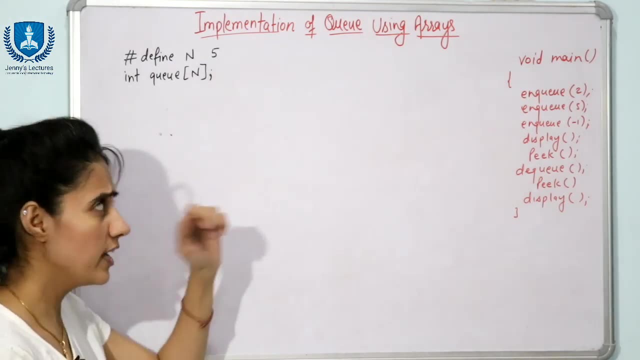 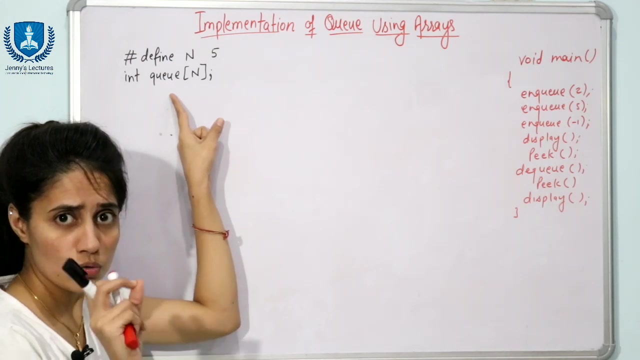 definition: hash define N- 5.. So in program, wherever you will use N, then it will replace this N by this 5. or here you can write: hash define: max size is 50, 100, like this right. but if you declare this queue size within these functions, then you: 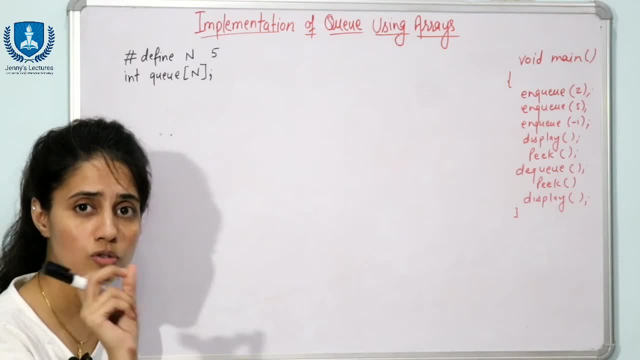 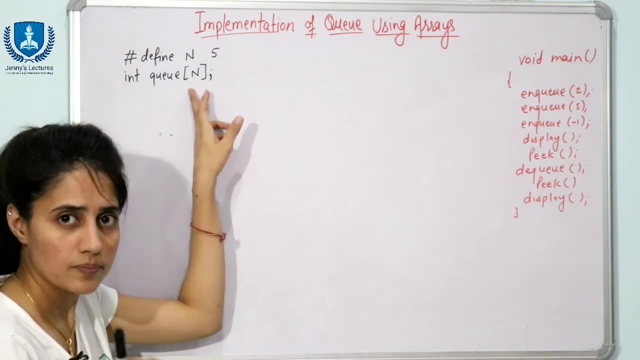 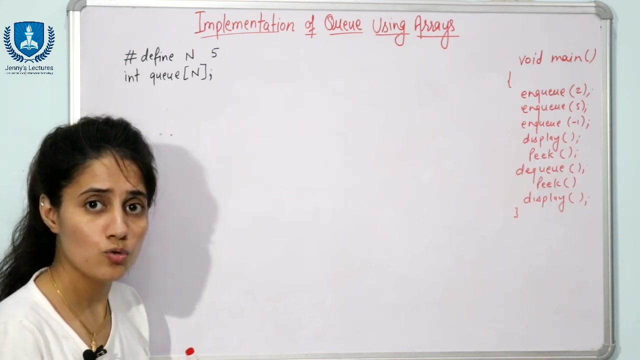 cannot write here the variable, then you have to specify here the constant term, either 5, 10, 50, something like this: right, I am declaring globally. that is why I can write here: N fine Now. front and rear in queue. these are two important parts that we have discussed. So you have to take two variables. 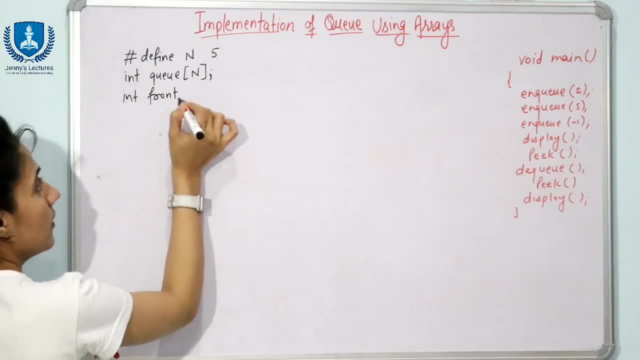 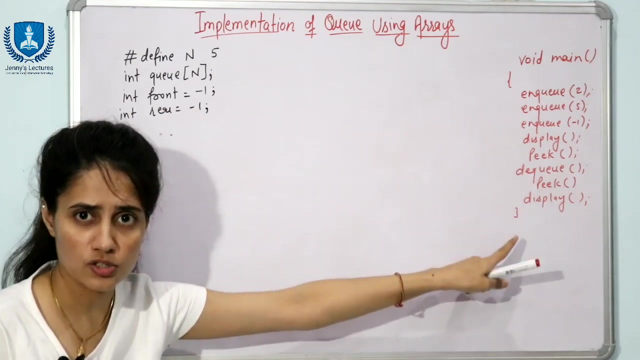 one is front and we will initialize this front first of all with minus 1 and rear is equal to also minus 1 globally, because front and rear both the variables we will use in each function. that is why I am declaring these variables globally, so that we can access these variables in each function. 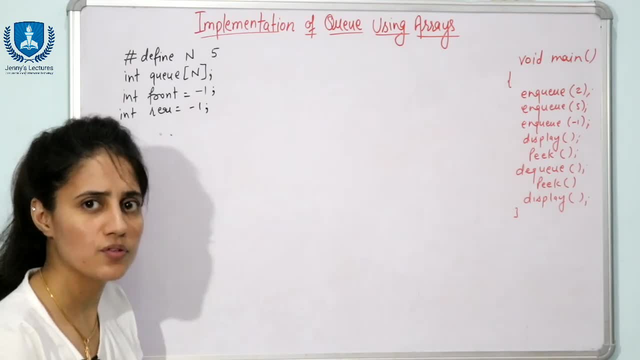 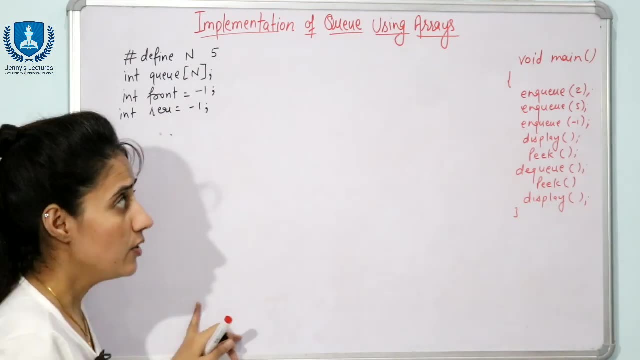 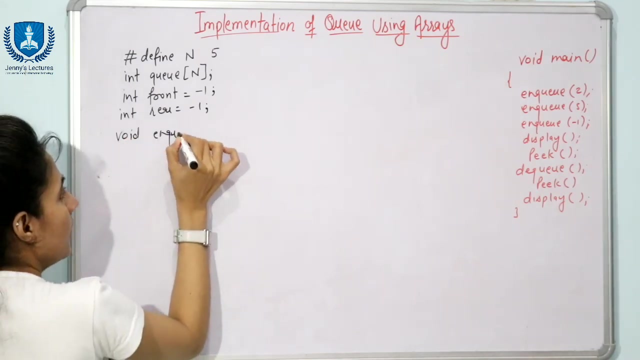 rather than declaring Those variables again and again in every function. right, and minus 1. minus 1 means queue is empty. we do not have anything. Now we are going to define this N queue function, right, how to write down the code? So here also see: here I am passing value 2, so obviously you have to receive this value. 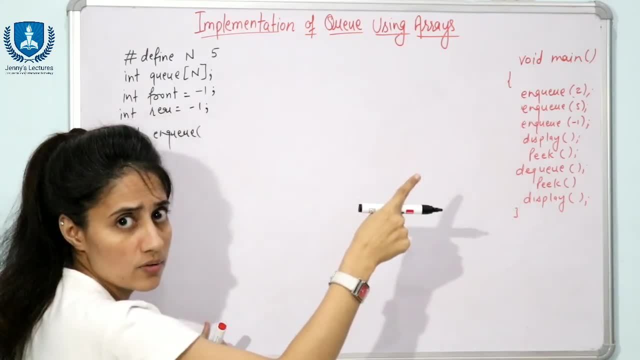 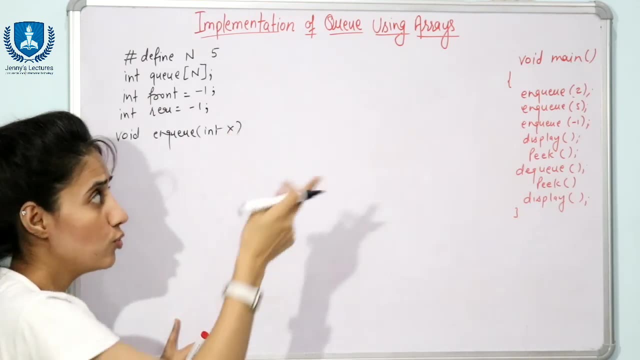 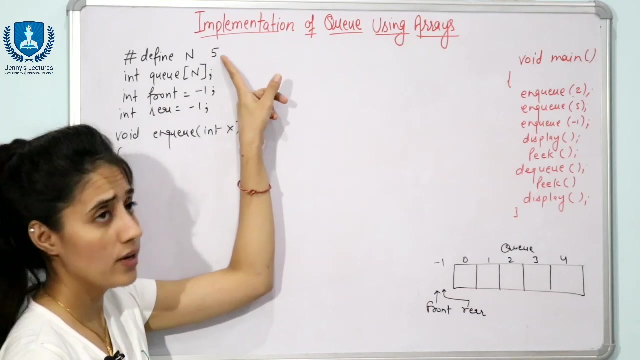 when you are going to define this function right here. I am calling this function fine. So now the data type of 2 is integer, I am going to take int variable to receive this 2 right. So you can say: this is the logical representation of this queue. Size is 5, N value is 5, 1, 2, 3, 4 and 5. this is actually an array, but we are 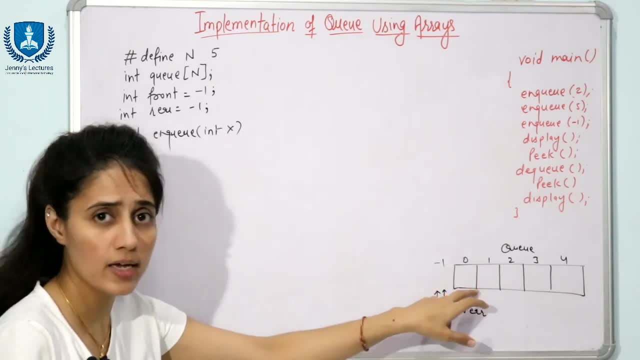 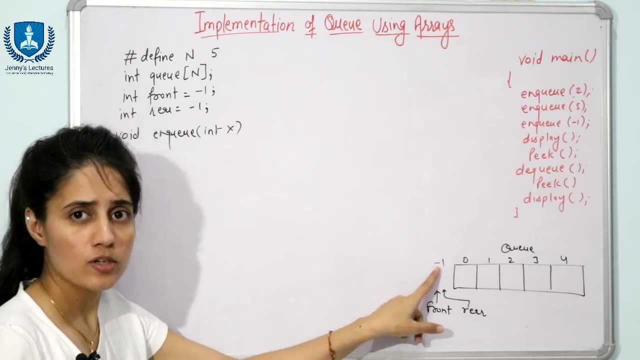 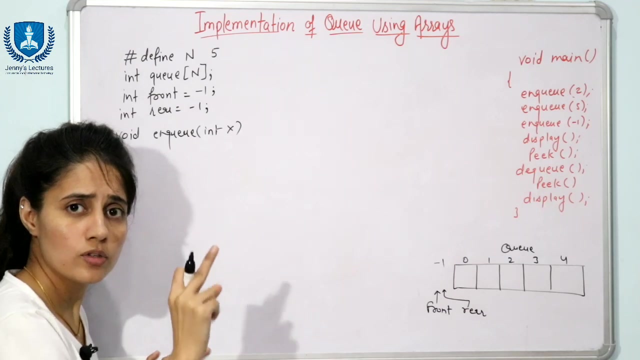 using this array for implementation of queue. So you can say: here I am using this array as a queue data structure, right, both front and rear, pointing to minus 1 right now. fine, Now see. first of all, you will check for the overflow condition, and what is that overflow condition? we have discussed in the previous. 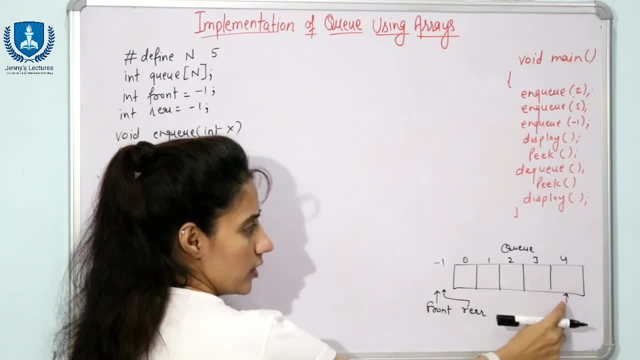 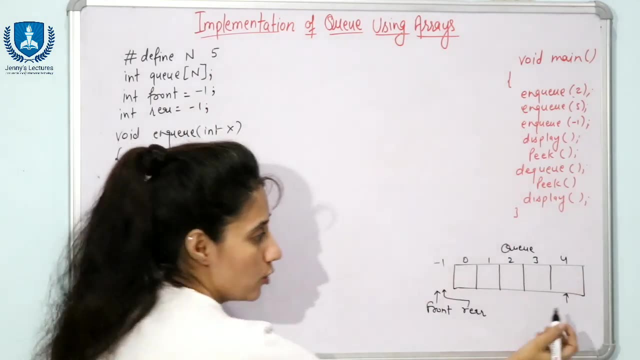 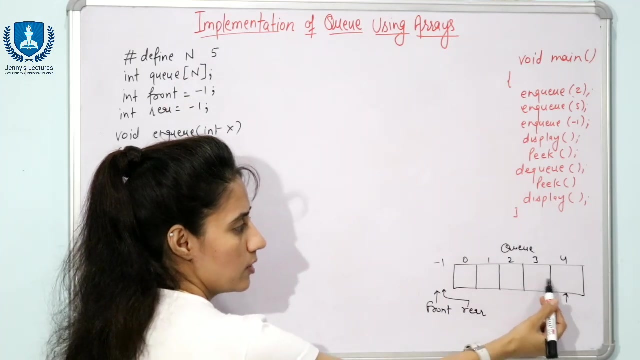 video: When rear becomes here. rear is pointing to here 4 means this: N minus 1, maximum size minus 1, because we will insert from the rear. when you will insert first element, then here it would be inserted means rear plus plus, then again rear plus plus, rear plus plus, rear plus plus and rear plus plus. 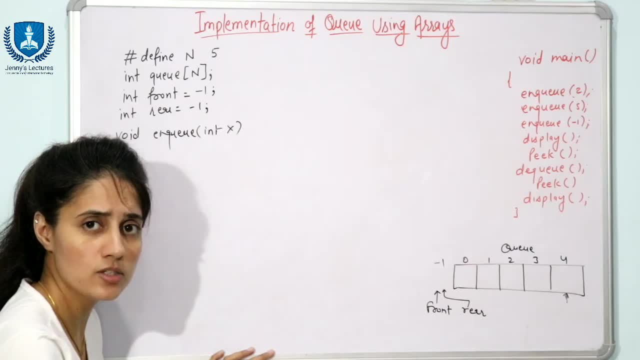 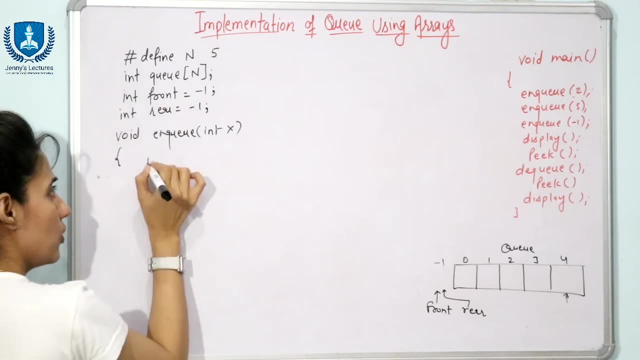 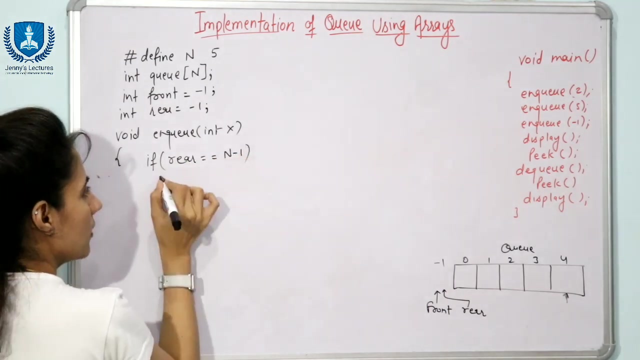 plus When rear is reached to here maximum minus 1, it means we cannot insert any other data here. queue is full. So first of all you will check for that thing for over overflow condition. Now, here you will write: if rear equal to equal to N minus 1, it means here simply you can print print. 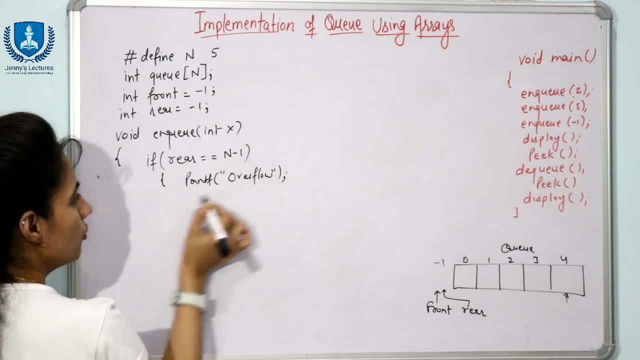 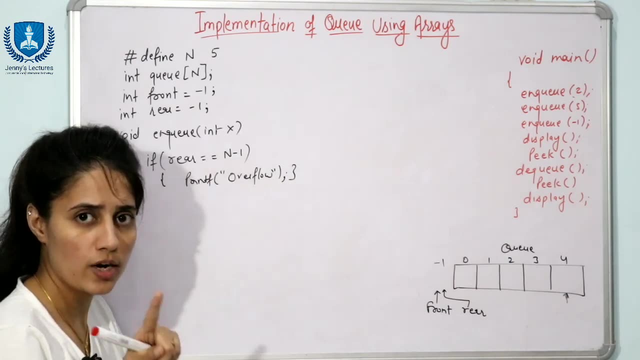 F overflow or you can say print F: queue is full right. This thing we have discussed in detail in the previous video. you should check out that video first. right Now this is not a case. so second case is when we as if there is nothing In the queue, like this, it is empty, then both front and rear would 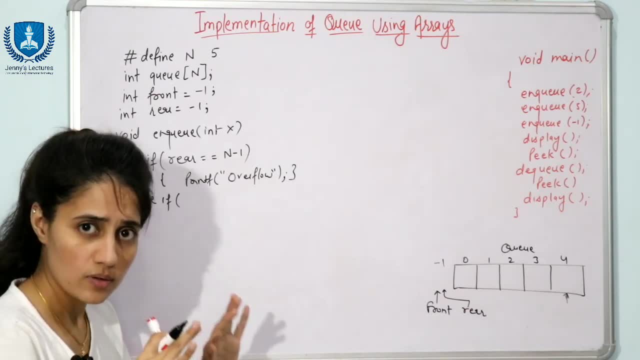 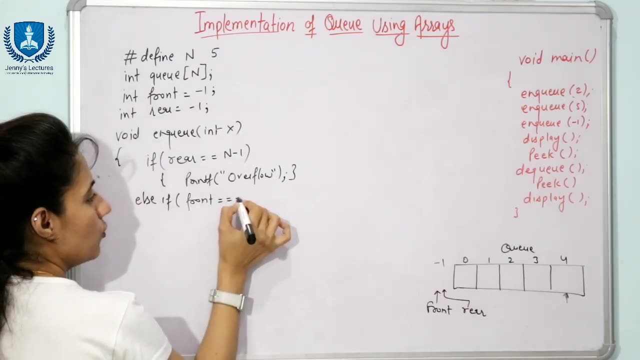 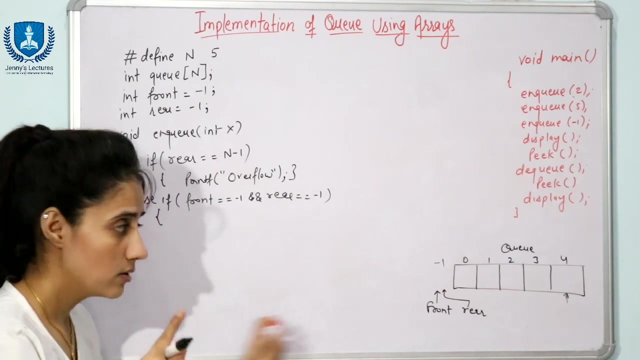 point minus 1. that is the condition we have ah considered for MPP queue. right. so now else, if Front equilib怪 to minus one and Real equal to equal to minus one, in that case do is impP T. now what you have to do first, we will insert the. 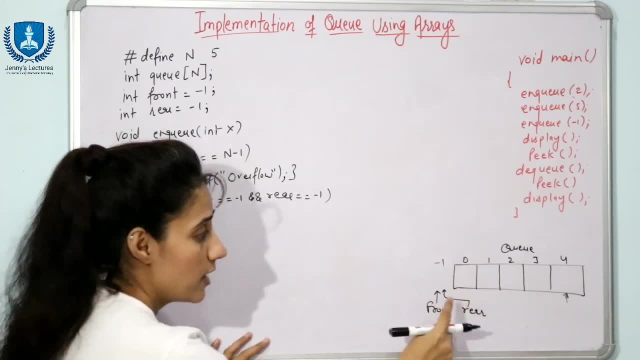 In the row after the orientation Results: Insert Thisraw pink: 介20はいisubt lleva� сторону HE哌aw, followed by ENforce yaw here. so front would be increased as well as rear would be increased. both would be increased right. 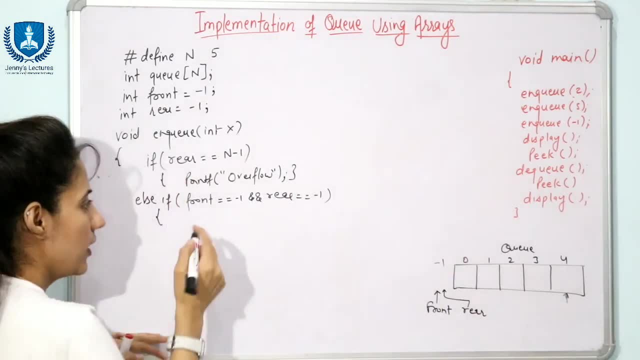 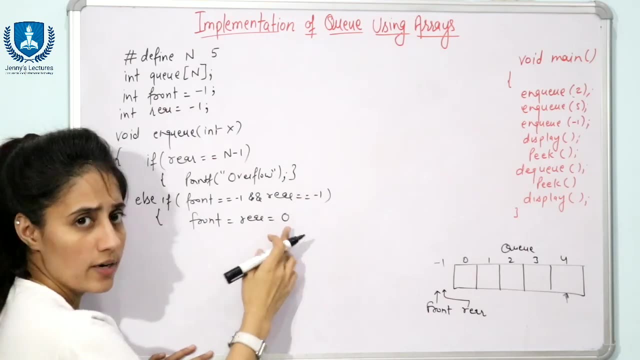 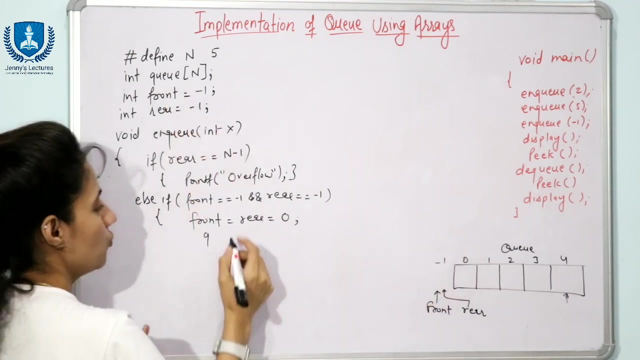 now both would point to 0. now here, simply, you can do: first of all, front is equal to rear, equal to 0 minus 1. after that it would be 0 after incrementing. so now you can insert here the data. so here what you will write: see the name of array we have taken is q. 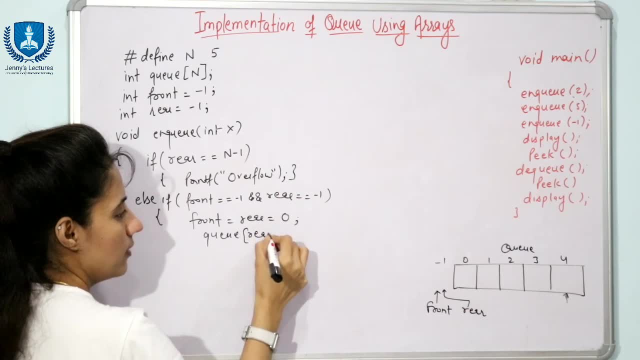 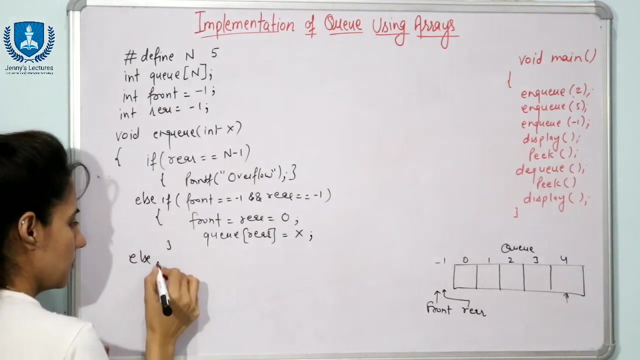 q and here you will write rear, because always we will insert from the rear. nq would be from the rear part is equal to whatever the value in x right now. third case may be else see. first of all, nq. 2 at starting q is empty. if rear equal to, equal to n minus 1, that this 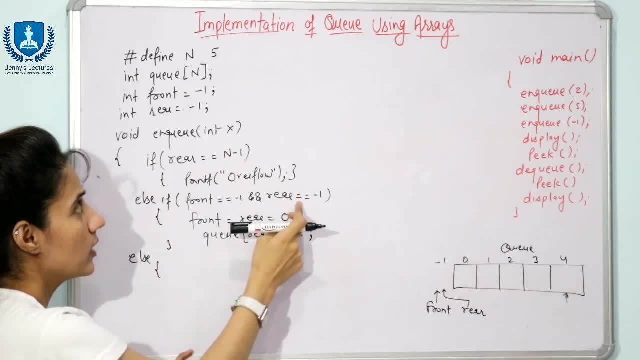 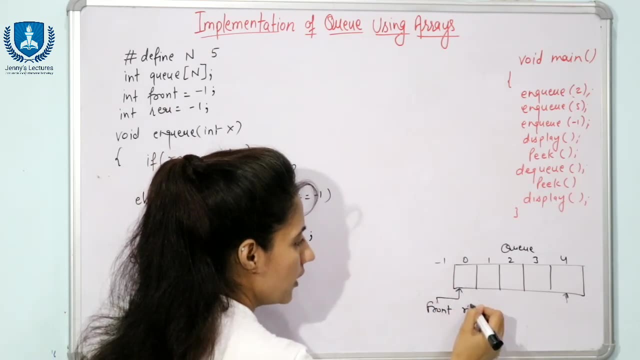 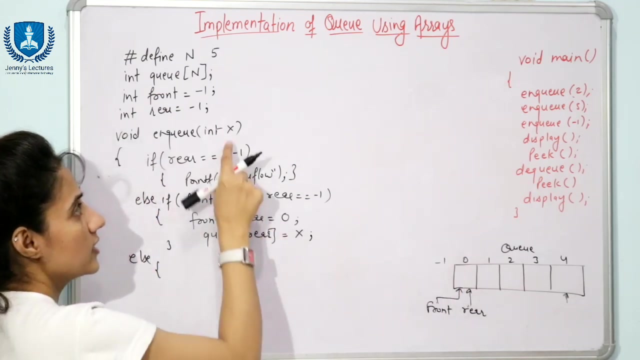 condition is not true. but this condition is true. front is minus 1, rear equal to 0 is minus 1. yes, both are minus 1, right front and rear equal to 0 means front is pointing to here, rear is also pointing to here. q of rear. rear value is now 0. q of 0 means here you will insert x, x. 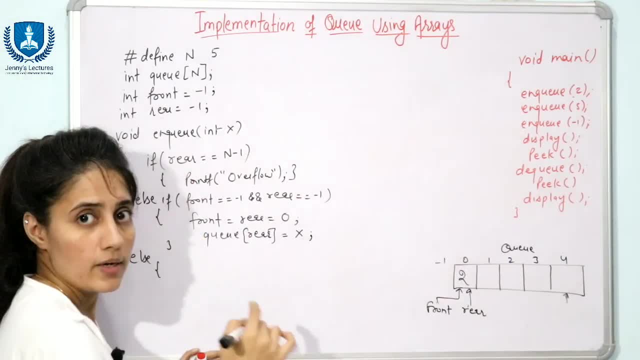 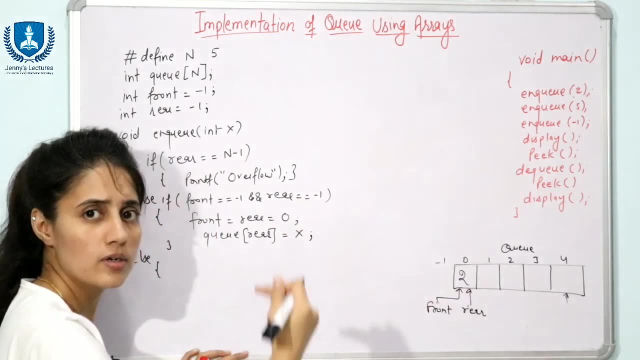 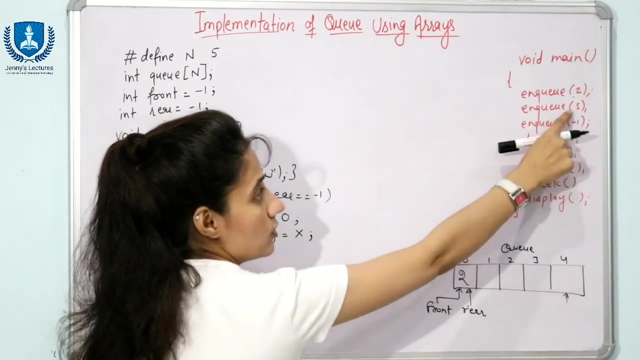 value is what 2? so now, here i have inserted 2. now, third case may be: q is not empty, q is not full, q has some data and after that i want to insert another data. in that case, what you will do. suppose i have 1 in this q, that is 2 i have inserted. now i want to insert 5. in that case, what you will do. 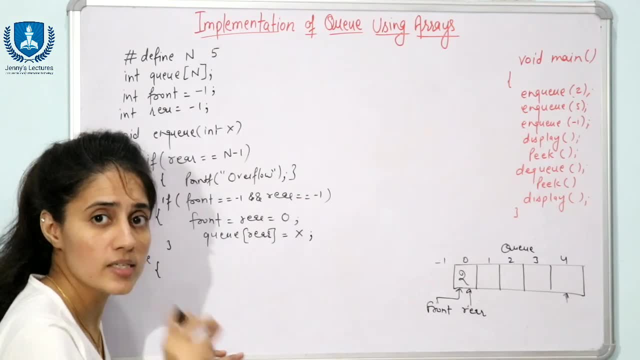 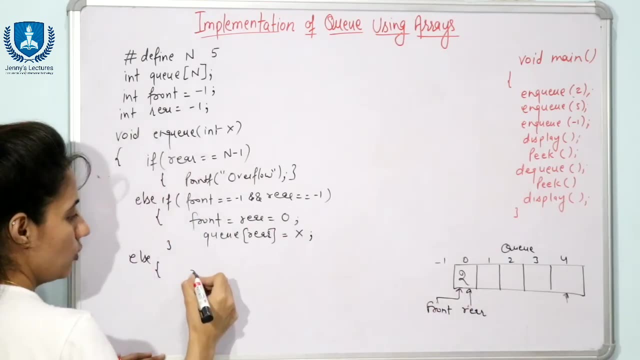 we will not touch this front because we will always insert from the rear end. that is the rule of the q right. so now, first of all, rear plus plus. so here what you will do. rear plus plus means rear is now pointing to here 1. now you can insert here the data. so 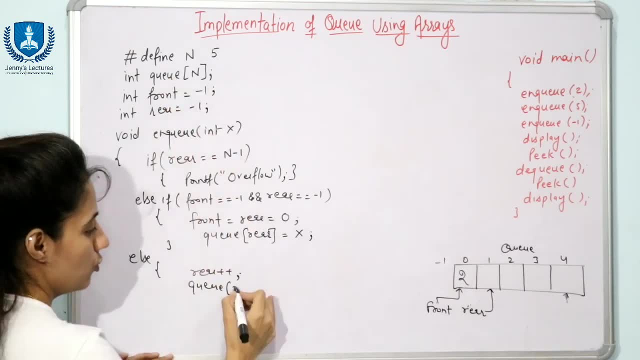 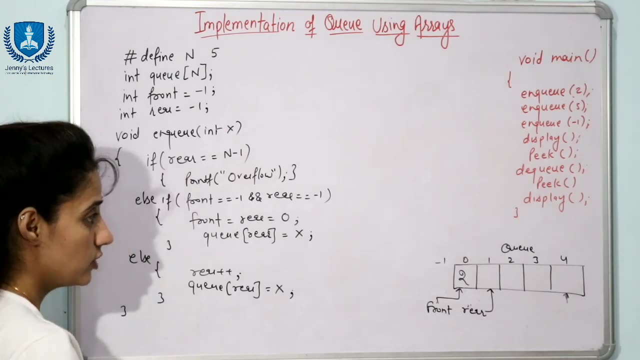 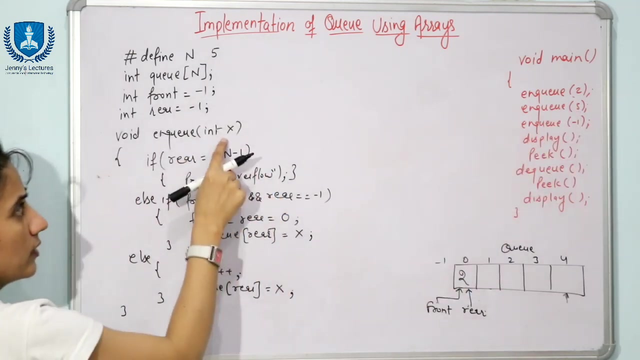 q name is q, q, q, q of rear equal to x. that's it. see, you can check. now after inserting to both rear and front would be pointing to 0. now again call nq function, nq 5. x now become 5 if rear equal to n minus 1. 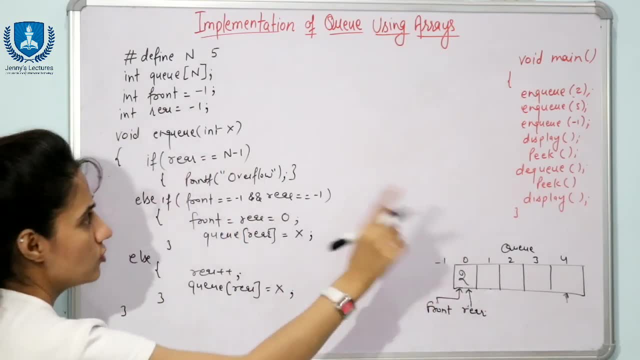 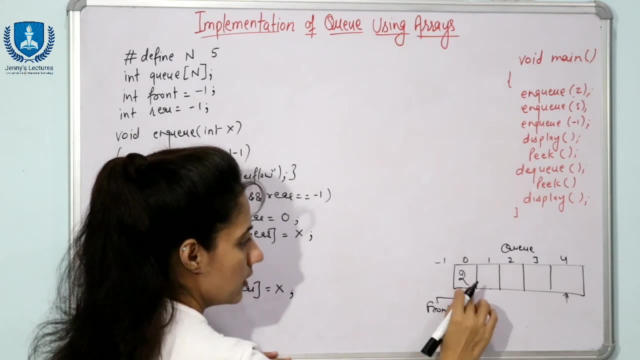 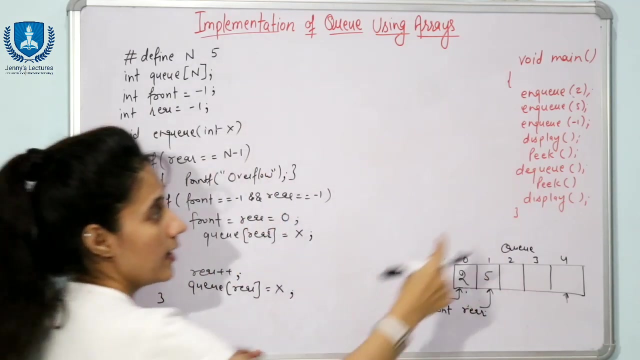 no, this condition is not true, because rear is 0, rear is not 4. this condition, this condition is also not true. now control will go into else part. rear plus plus means rear. would be pointing to here now q of rear, q of 1 is equal to x. now here we can insert 5 again. call nq minus 1. 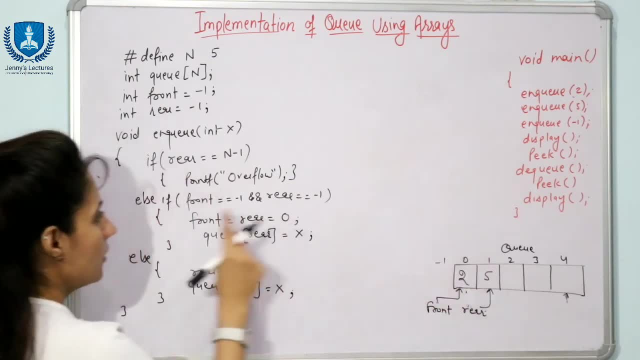 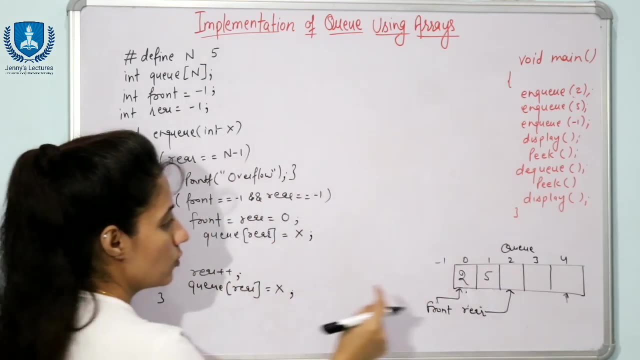 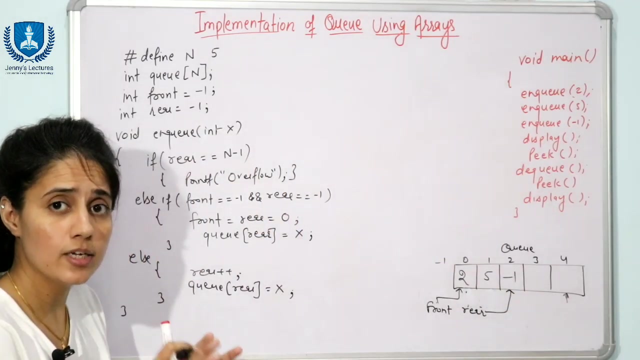 this condition is not true because rear is still 1. this condition is also not true now rear plus plus. now rear is pointing to here. rear becomes now 2. q of 2 is equal to x, q of 2. here we will insert x. x value is minus 1, so this is the nq function. now we will see the decoding for. 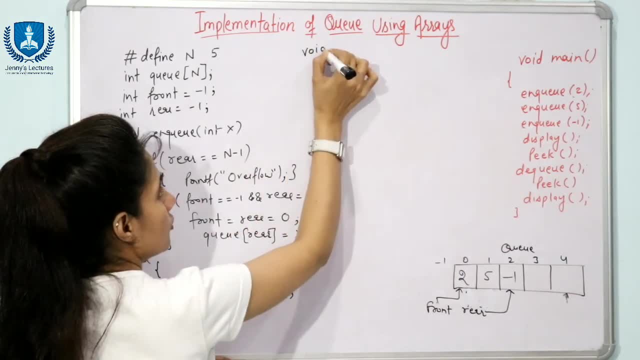 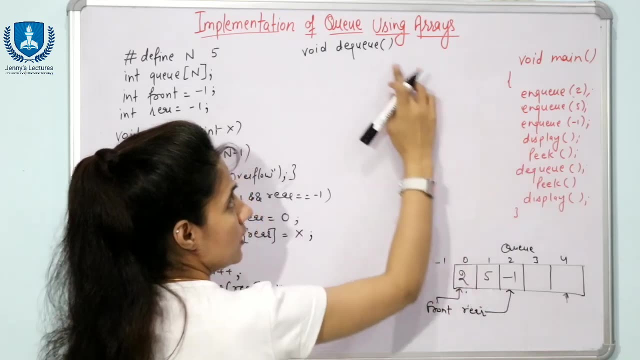 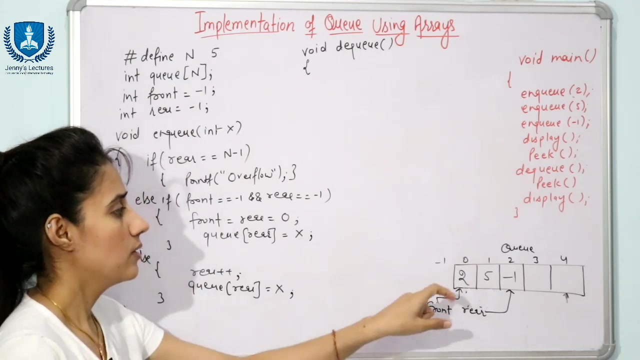 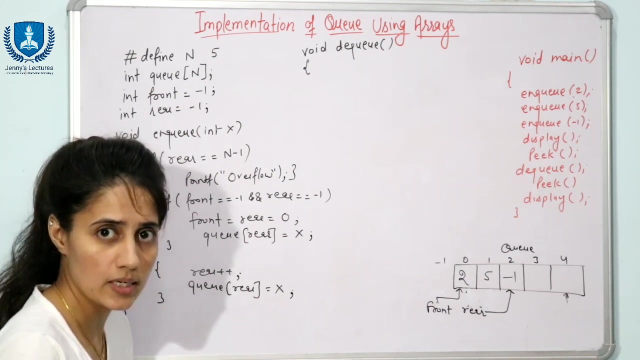 dq function. right here i am writing this dq function. you nothing. we are see dq function. we are not passing anything, so i will not write anything here. right here also some cases are there first cases: if the this q is empty, in that case dq means: can we delete anything? no, we can't delete anything, right, so first you will check if 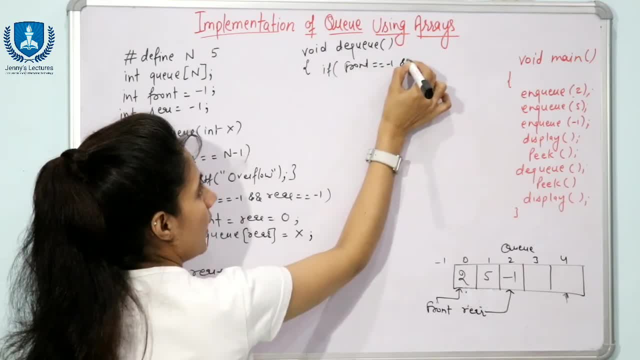 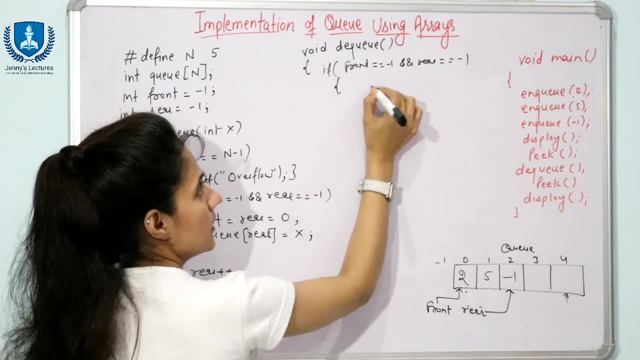 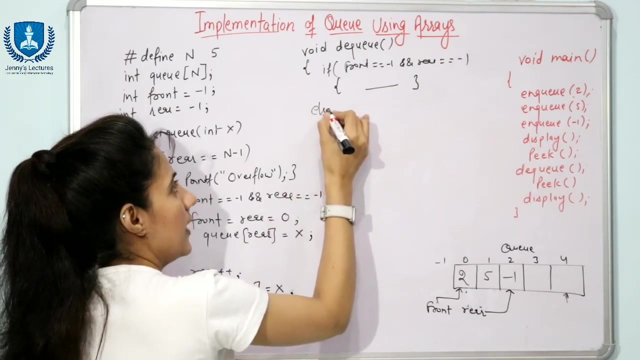 front equal to equal to minus 1 and rear equal to equal to minus 1. this is the condition of empty q, right? in that case, here, simply, you can print what list Plant gossip which is empty, or you can say underflow point condition. now else, if when both front and rear, 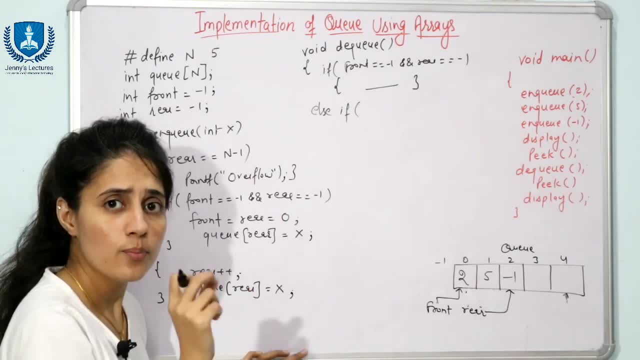 are pointing to the same index. this thing also we have discussed clearly in detail in the previous video, so you should check out that video. first of all, suppose i have called dq function two times and dq means i have deleted this. i have deleted w and this q very easily, because this will close out all that is this: i have creations i have targeted by few when dq failed and in second placerophe function two times and this is 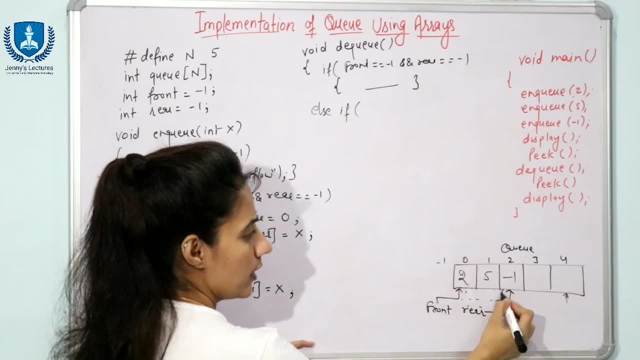 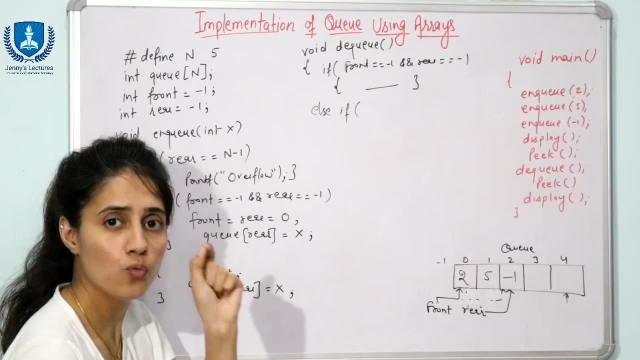 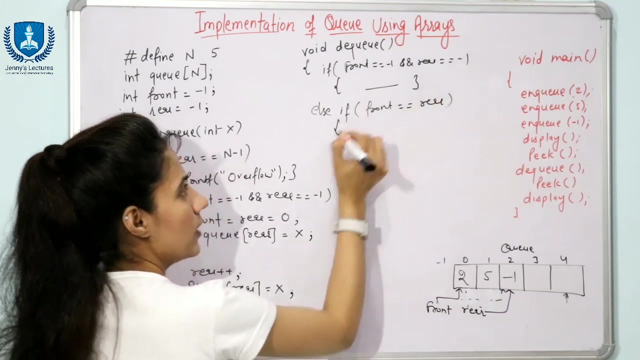 this, after deleting these two- front would point to here and rear is also pointing to here- means both front and rear are two. it means there is only one element in the queue. so here, if front equal to equal to rear, it means there is only one element. and after deleting this element, 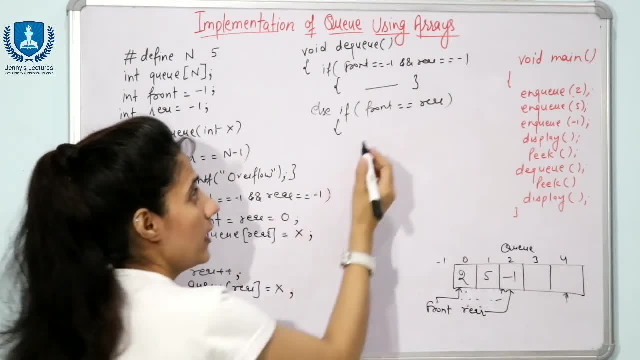 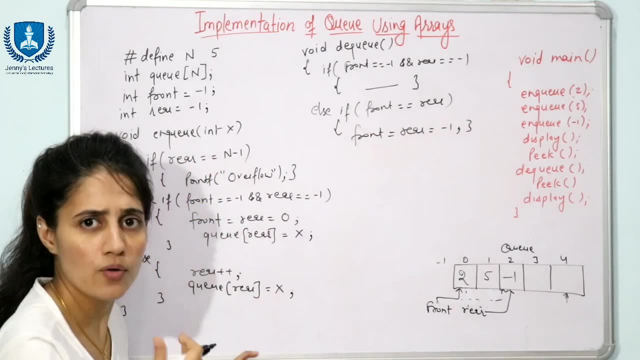 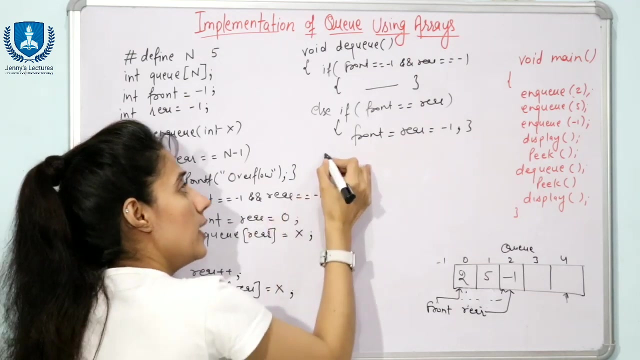 this queue will be empty, right. so here what you will write: you will set both front and rear equal to minus 1, because this is the condition we have taken for empty queue, for showing the empty queue, front is equal to minus 1, rear equal to minus 1, right. so that's it now. third case may be this case: 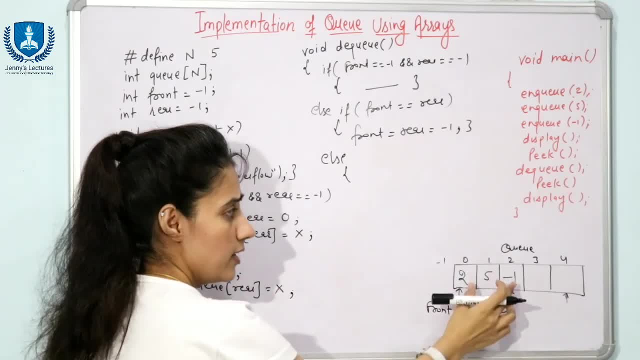 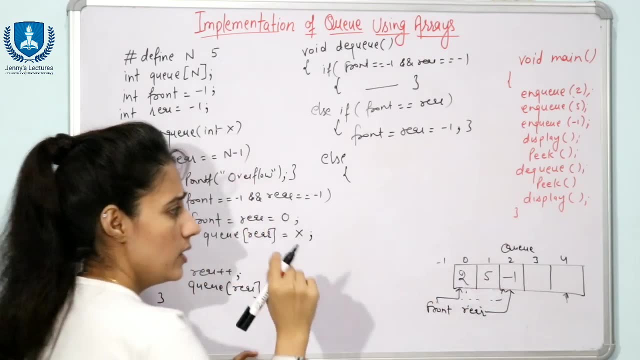 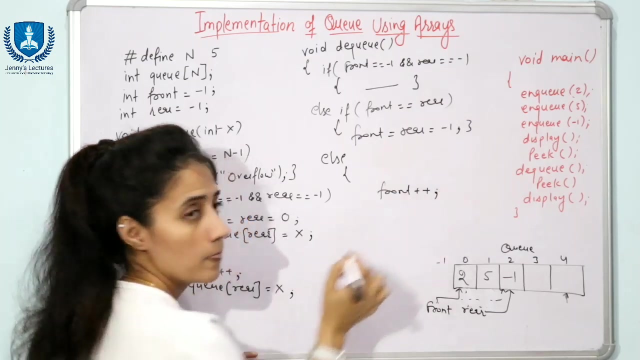 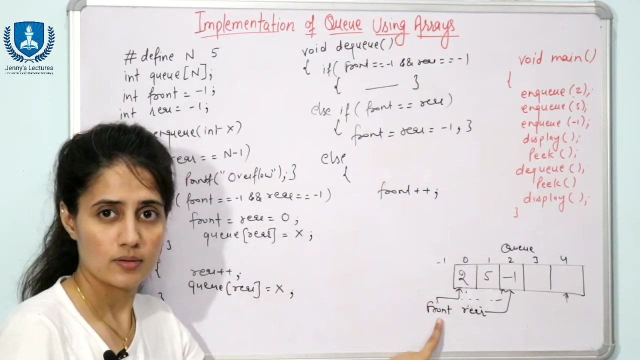 q is not empty and there is more than one element in the queue. in that case, what you will do? suppose we have three elements in the queue. now, simply, you will do what? front plus plus? here i can write front plus plus because dq operation can be performed on the end. that is front we can delete data from. 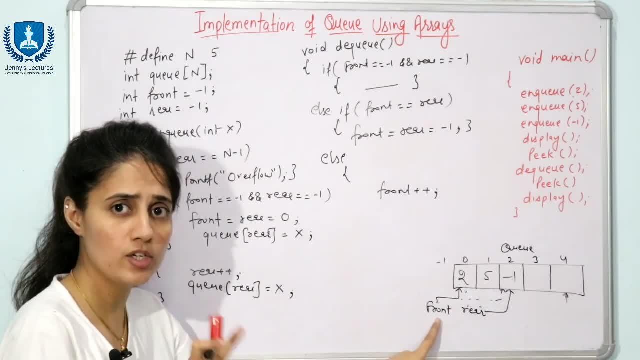 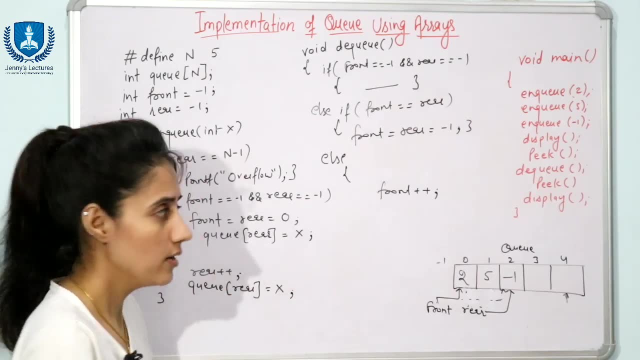 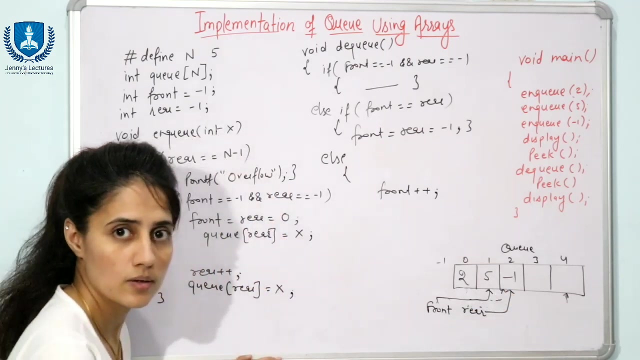 the front only. that is the rule of the queue. you have to take care of these rules right, because we are implementing here q, so you have to enforce these rules here, right. so front plus plus. front plus plus means now. front is pointing to here, right now. this is what a garbage. 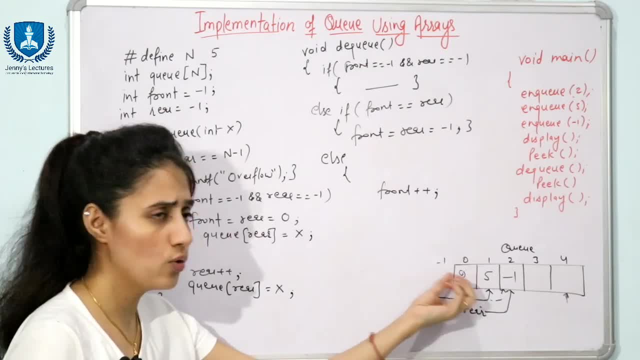 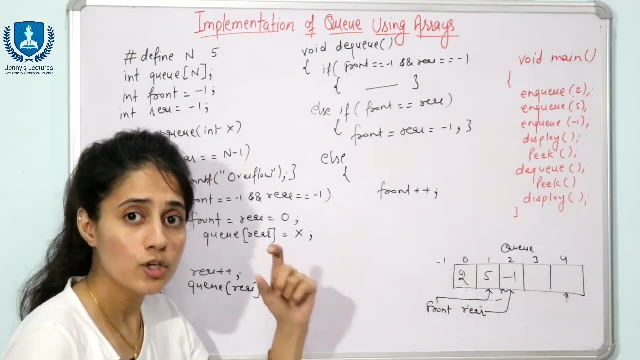 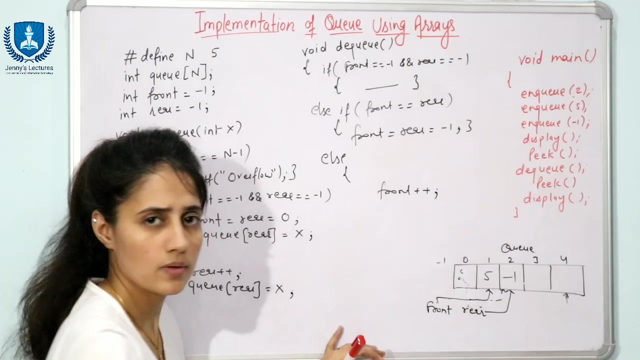 value means we don't care what garbage value lies here in this cell, because suppose in future you will access this cell, then you can overwrite this value. the q is basically from front to rear means this is now the queue. so this is now a garbage value for us. you can delete it, right. 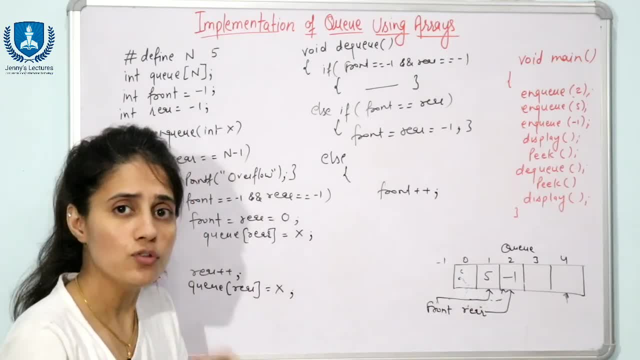 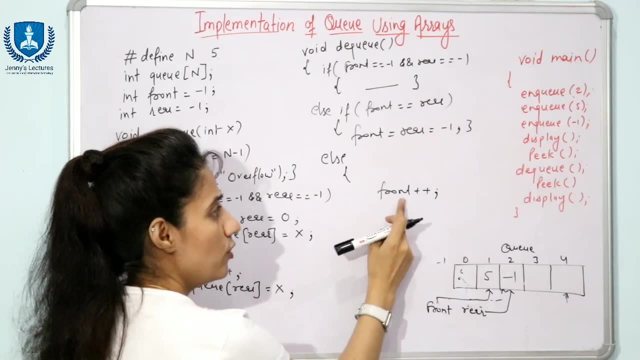 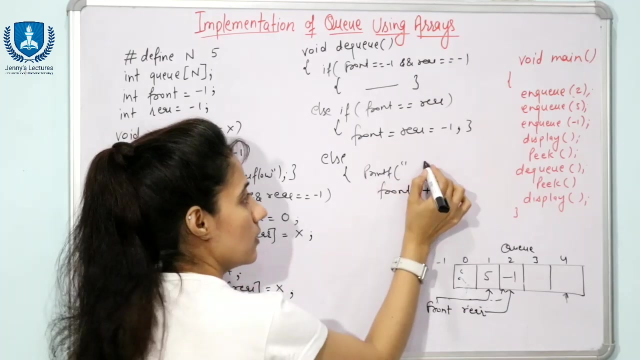 simply you have to do front plus plus and that's it. and if you want to print the dq element, you want to check out what element you have dq, then before doing front plus plus here you have to think about while writing. here you can write: print f. the dq element from the q is percentage. 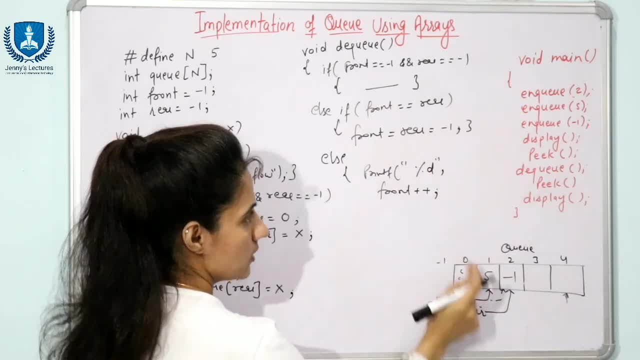 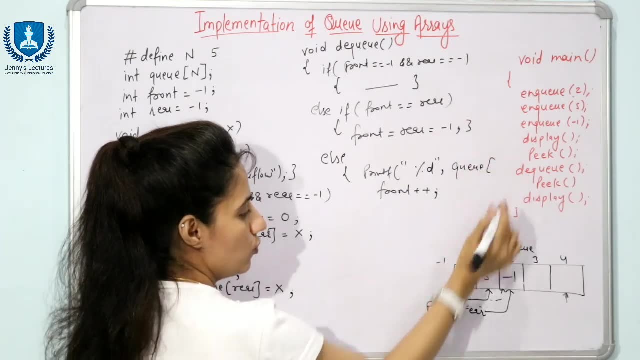 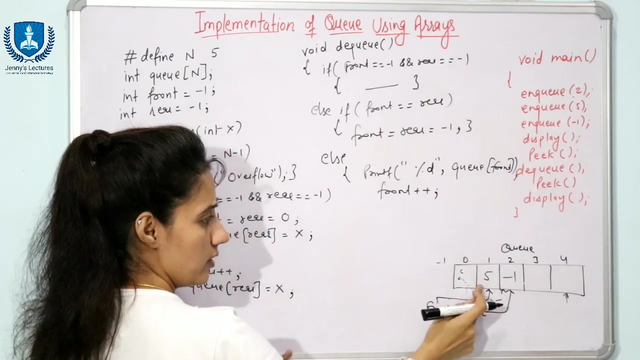 d. i am writing only this thing because i don't have space, so here you can print first of all this data. so how you will access this data, name of this is q, q of this front, because before up, after, before updating this front, front was pointing here. q of front means q. 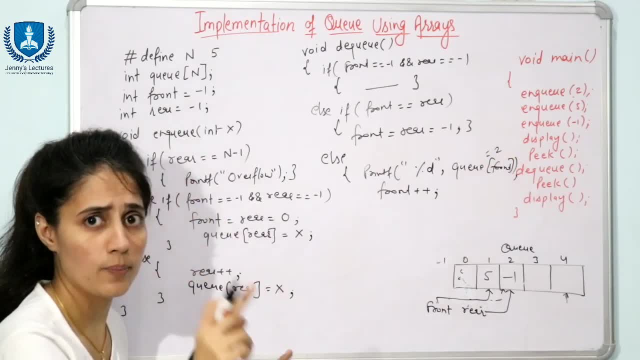 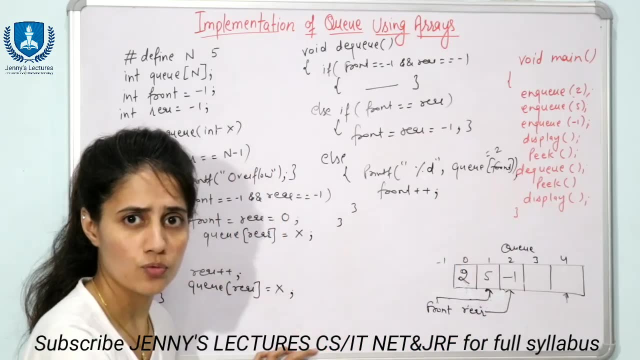 of zero, this would print two, and after that you can do front produce 0, and after this you can do inside, print k, 0, and after that you can do front produce 0, and after that you can do inside plus plus. and that's it now. suppose again after this dq, again i am calling dq, right again control. 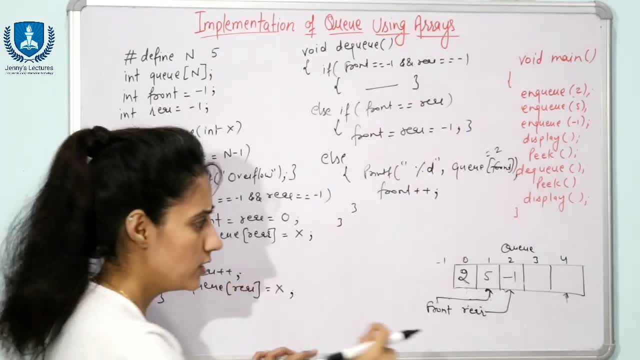 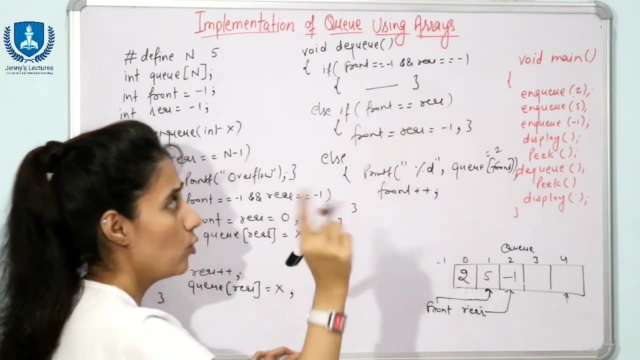 will go here. front equal to minus 1, rear equal to minus 1. no, this condition is not true, because front is 1, rear is 2, so control will not enter here in this loop else. if front equal to equal to rear. no, this condition is also not true, because front is 1, rear is 2, so control will go in else. 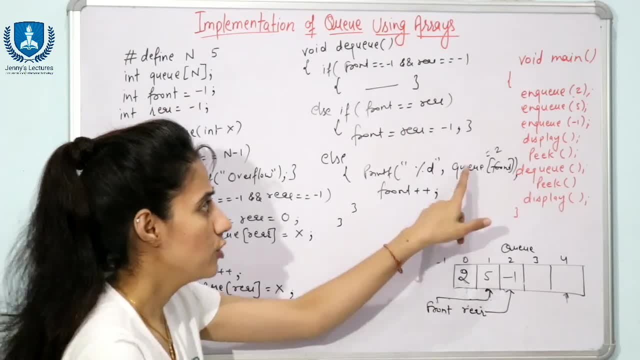 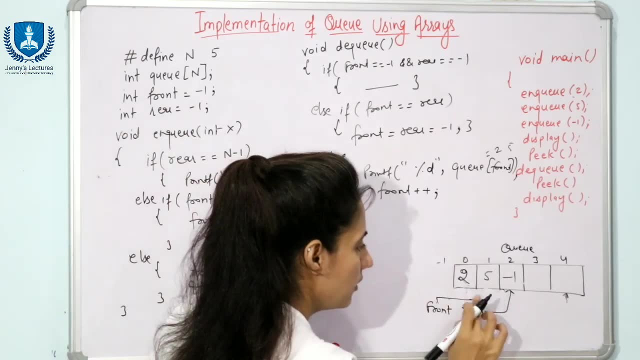 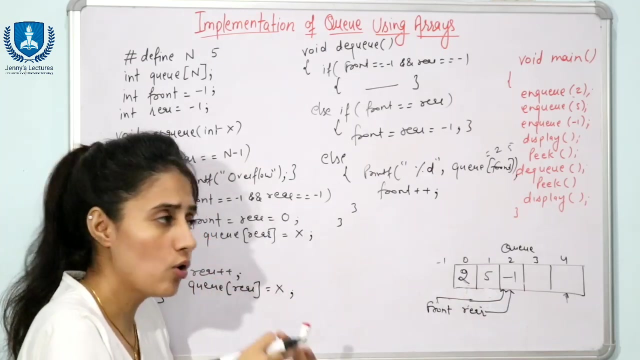 power print. if the dq element is q front, q front is 5, so it will print 5 after that front plus plus means after that front becomes here. 2 front would point to here. now again, suppose 3rd time we are calling q function. in that case what would happen? see now, see, this is the garbage value front and 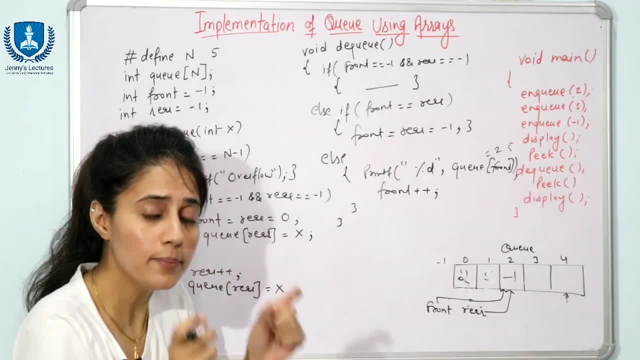 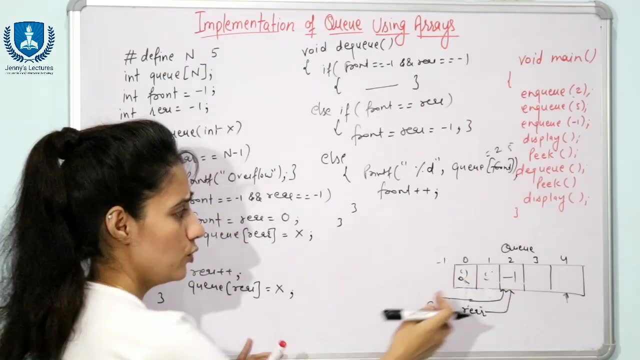 rear are pointing to here. so the q is only between front and rear. so this is only the q now here. so this is only the q now. so this is only the q now. these are garbage value means we have deleted these values. right, we don't care what values. 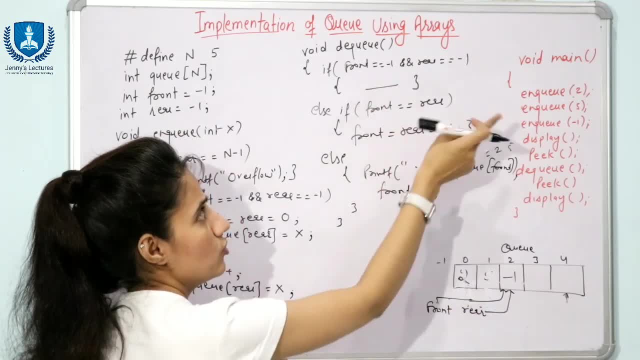 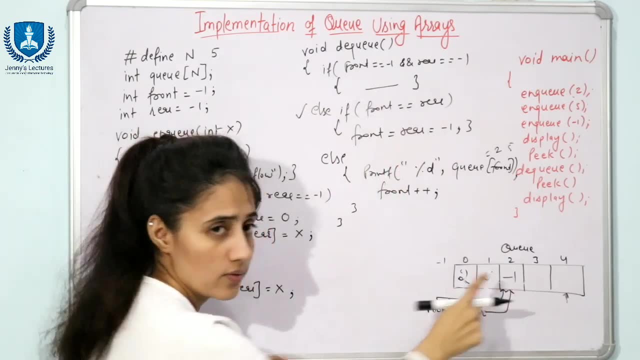 lies here. now, this condition, this condition is not true. this condition is true now: front equal to, equal to rear. front is 2 and rear is also 2, as you can see, right. so it means we have only one element and, as you can see, we have only one element left in the queue. so front and rear equal. 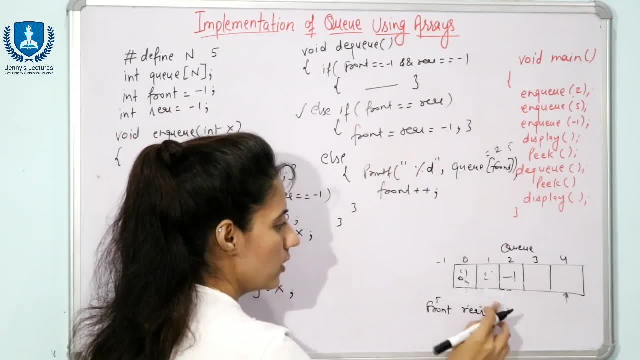 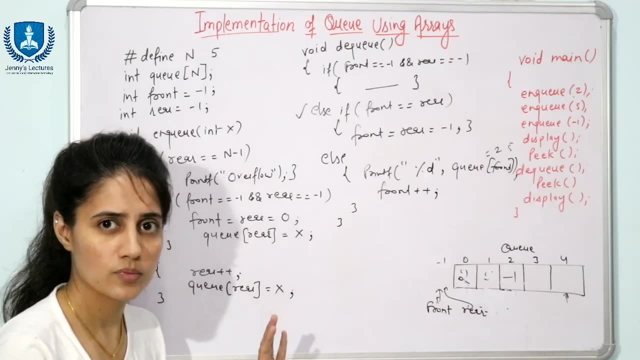 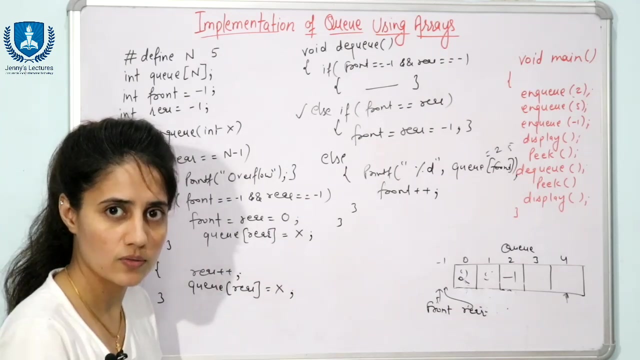 to minus 1. we will both set these- front and rear- equal to minus 1. both will point here. it means this is also now garbage value. we don't have anything in the queue, right? so this is how we are going to nq and dq the data. now. we will see the coding for display and peak function now at. 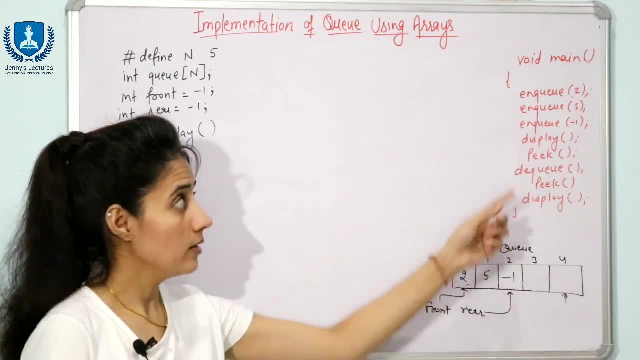 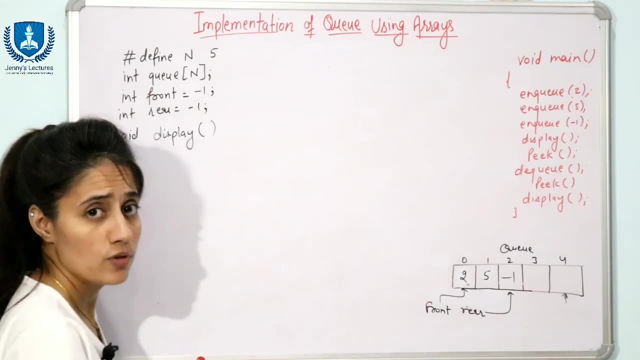 some point of time in q i have 2, 5 and minus 1, right after these nq function. now i want to display this data, whatever the value in the queue. so now i will define the display function. first of all, you will check if the queue is empty. in that case, obviously, there is nothing to display. 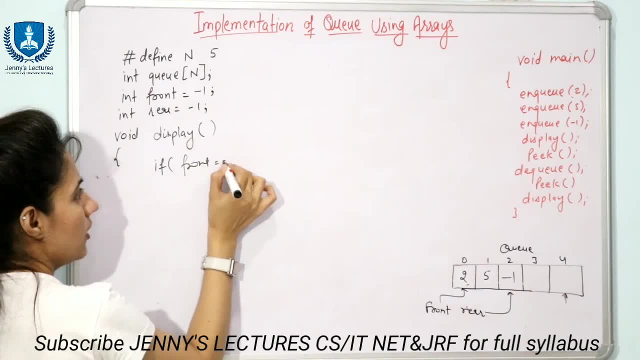 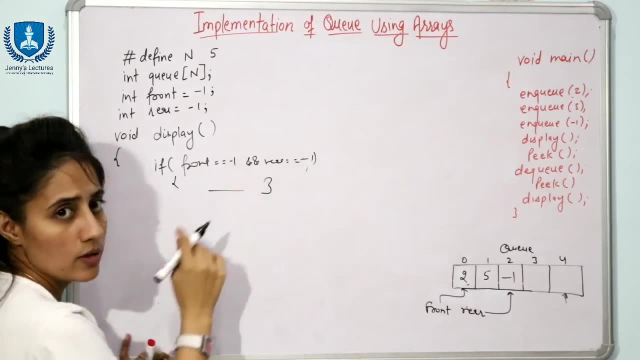 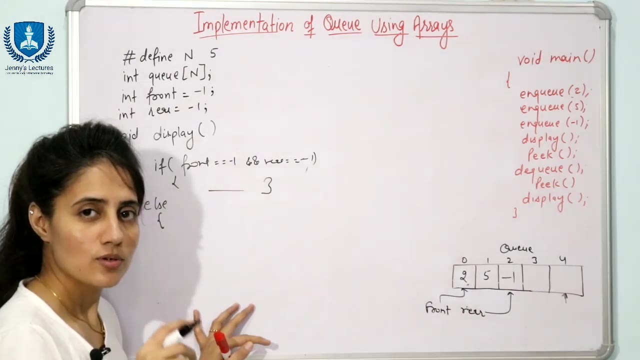 in the queue. so what is that condition? you will write: if front equal to equal to minus 1 and rear equal to equal to minus 1, in that case, here you will print what q is empty, right else, now we will print this data. see, every time i use 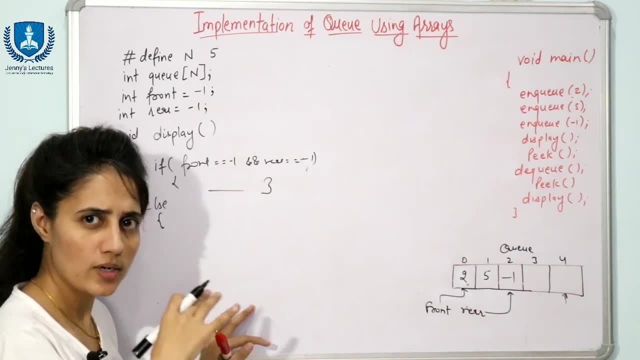 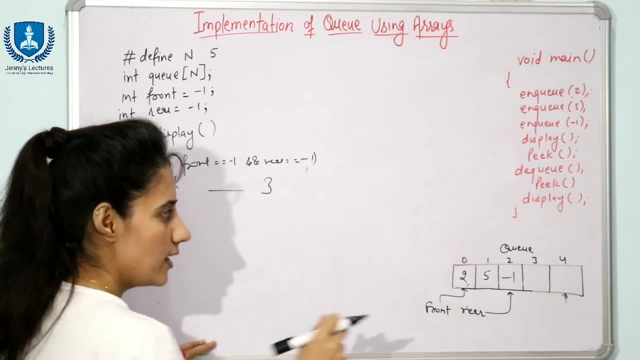 while loop when you are traversing the list or anything, or you are displaying the content. but someone asked me why all the youtubers use while loop. so in this video i'll use for loop. fine, so i'll display using for loop. so for that case else, 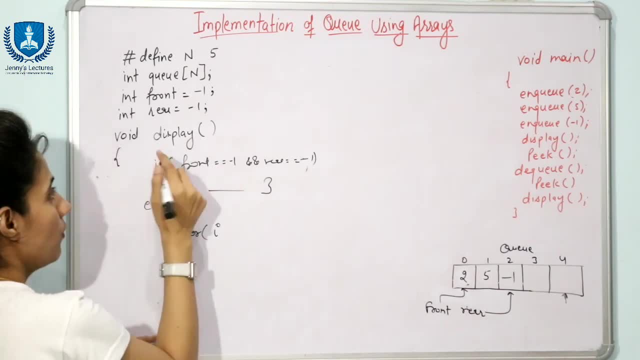 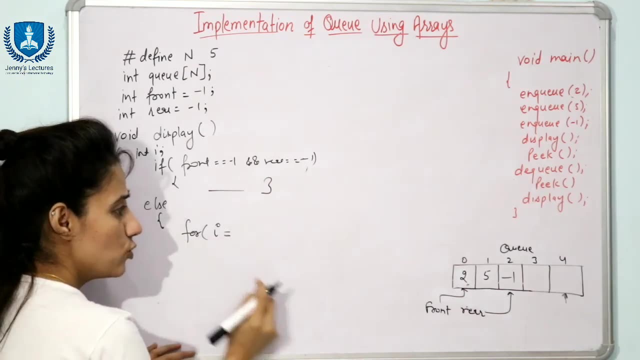 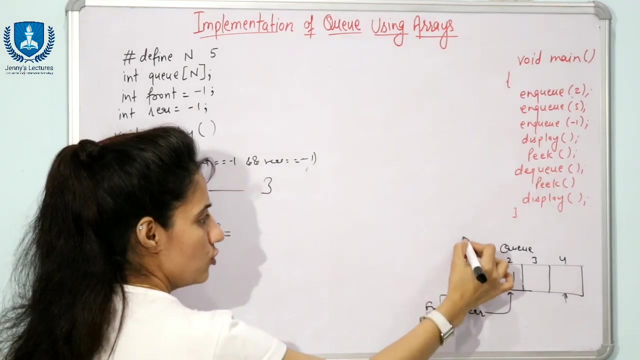 now, obviously you have to take a variable i, so you have to declare that variable i here in the display function, right? otherwise it will give you error. now, first of all, i is equal to front, from where i will display the content, that is 2, 5 and minus 1. so first of all i should point to here i: 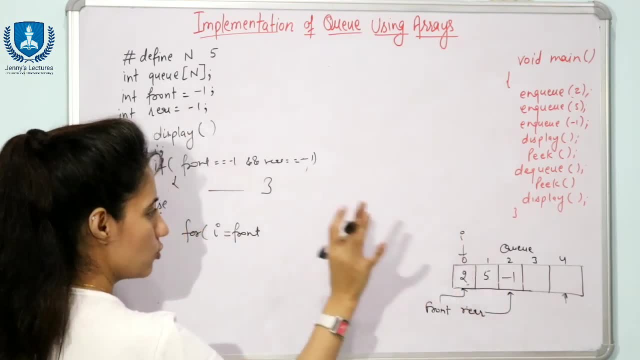 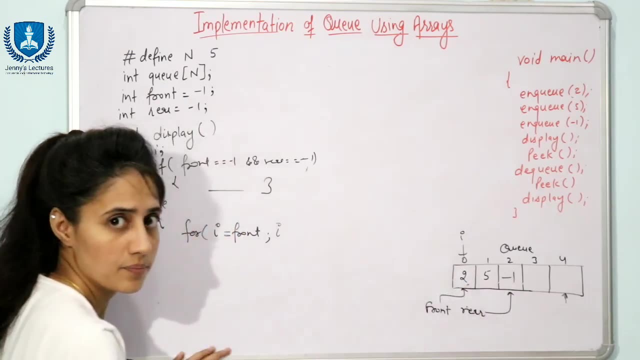 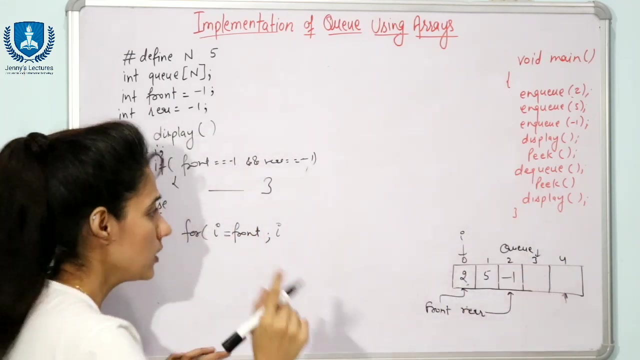 is equal to front. front is 0, so i is also 0 right now. we will move this i and print the data till here. right till here. i want to print the data. once i reach to 3, then i will stop. so here you can write. i'll print the data till i less than. 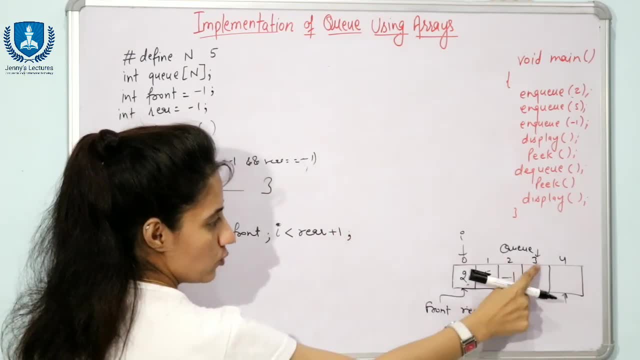 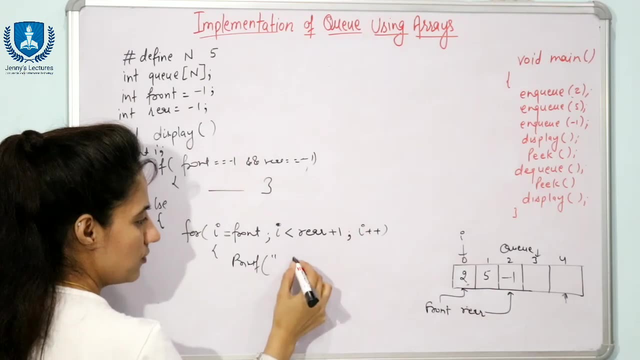 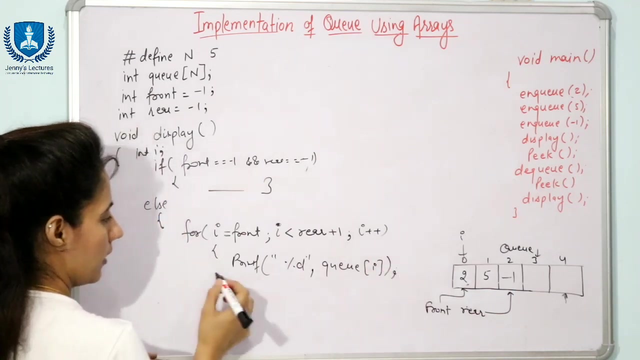 rear plus one, that is rear is two, rear plus one, that is three. till then i will do i plus plus and here i will print that data. so here simply write: print f, percentage, d and q. in subscript i will write i right here. in else part you can write the q is and after that you: 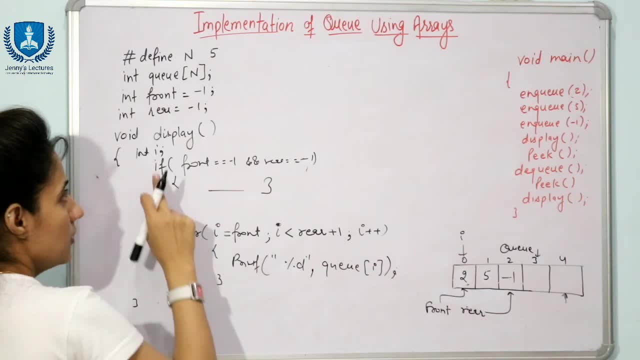 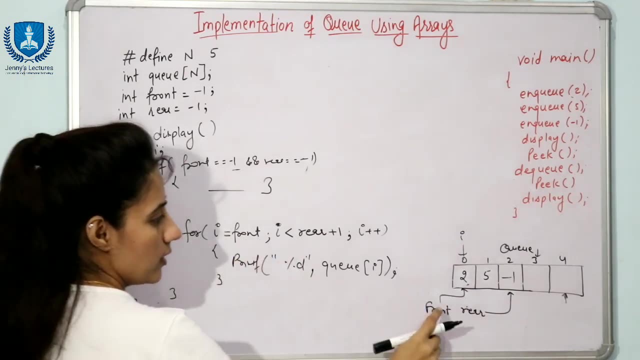 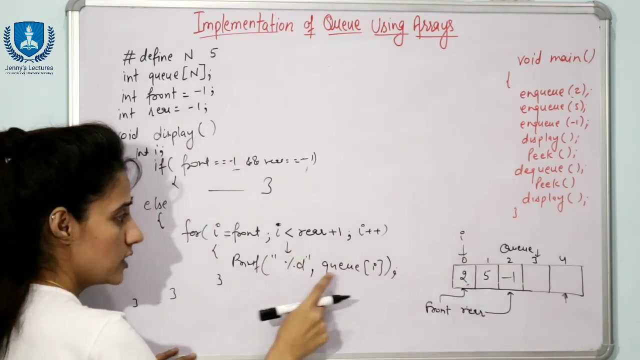 can print fine. now see see the working of this for loop. this is not the case, so control will go into else. part 4i is equal to front. front is 0. i is also zero, i less than rear plus one year. plus one is three. yes, condition is true, so control will go into this loop. percentage d: q of i. q of i means q. of zero two would be perfect because q is from bottom right. so so you can see that when you, if you take q here, you can print 4, so control will go into this loop. percent is dq of i, pure weight. here is what this x hat, because i mean q of 0, 2 would be 0 of 0, 2 is going to. 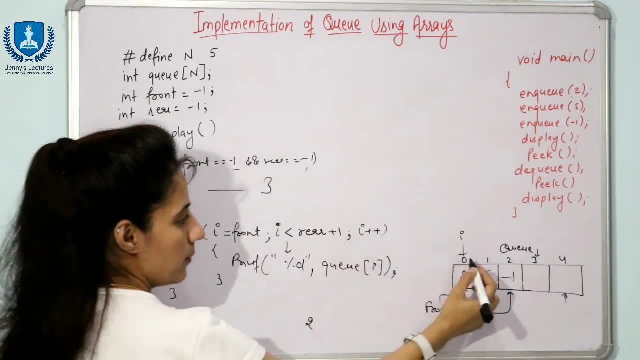 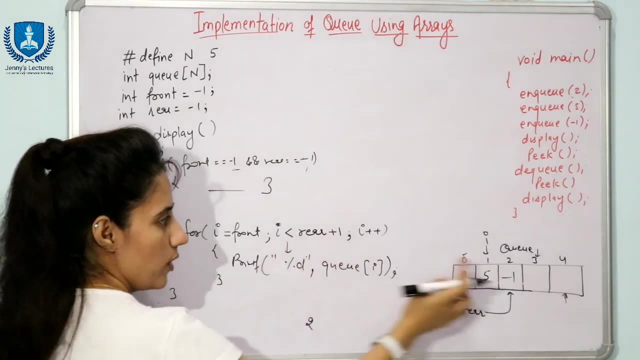 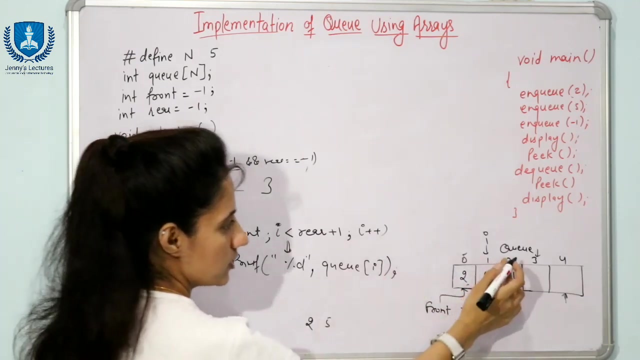 be printed right. i plus plus, now i becomes 1. i is pointing to here, now i is, containing value 1: 1 less than rear plus 1, that is 3. yes, control will go into this loop again. q of 1 would be printed. q of 1 is 5. 5 would be printed again. i plus plus, now i becomes 2. so here is i, now i is. 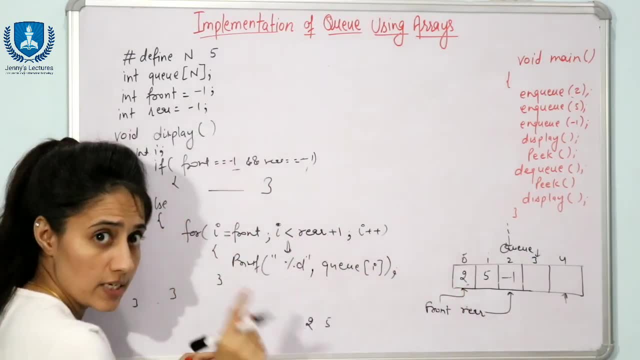 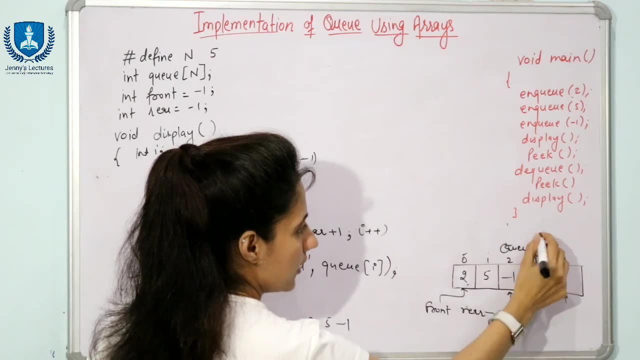 2. 2 less than rear plus 1. rear plus 1 is 3. yes, condition is true. again, printf q of 2, that is minus 1, would be printed i plus plus. now i becomes 3. so i is here now 3 less than 3. no condition is. 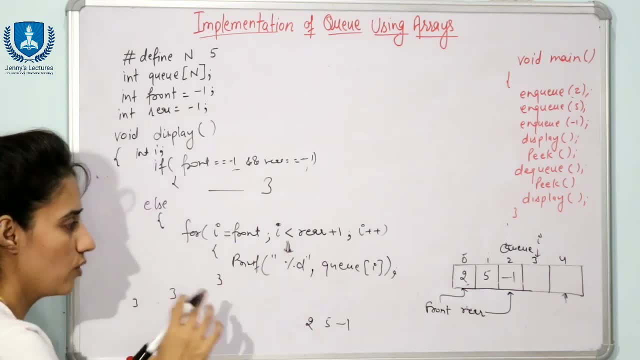 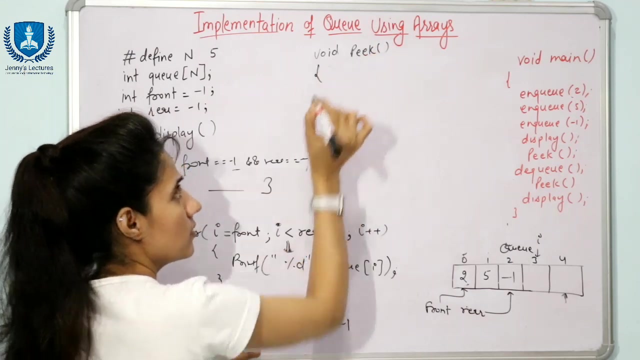 not true, so we are not going to enter into this loop. now exit from this loop. right? so the output is 2, 5 and minus 1, right? so this is what our display function, now the peak function: how you will write that coding. this is very simple. we are just checking what the value here at the front of 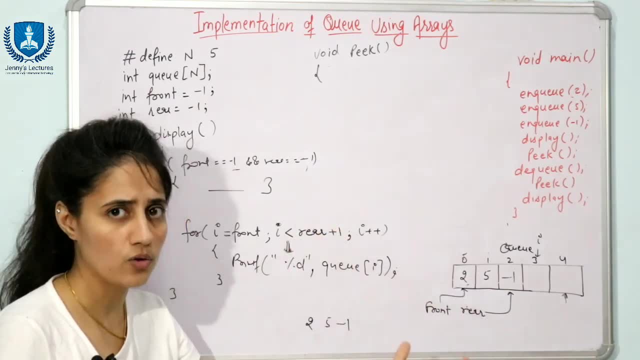 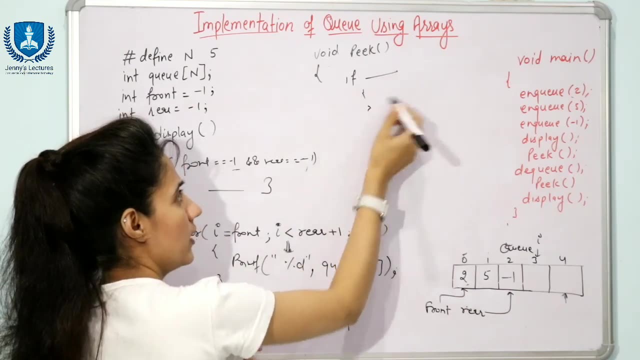 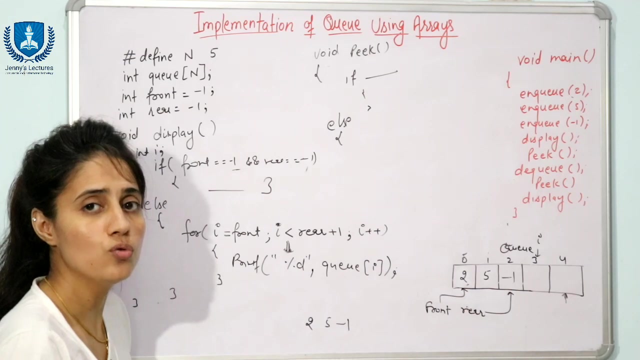 the q. what is that value? right, without removing that value in peak. also, you can write down this condition for checking the empty queue, right? i guess you can write down this condition. i am not writing this in else part, what you will write now. if condition now the q is not empty, in that case you have to print that data. 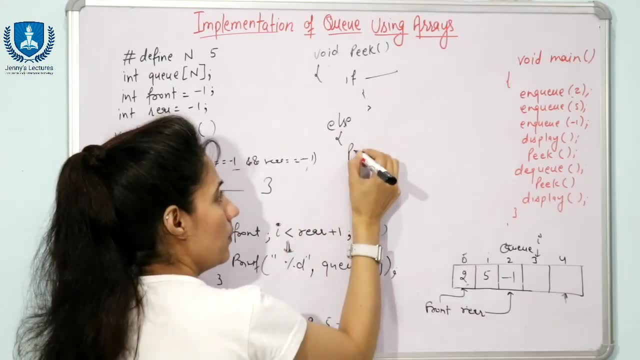 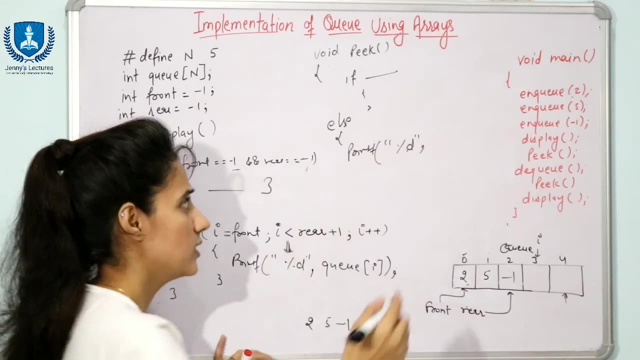 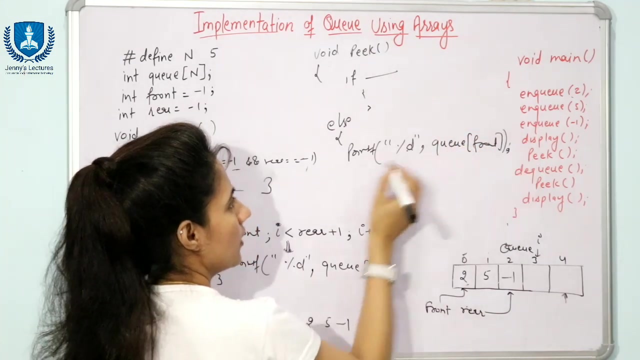 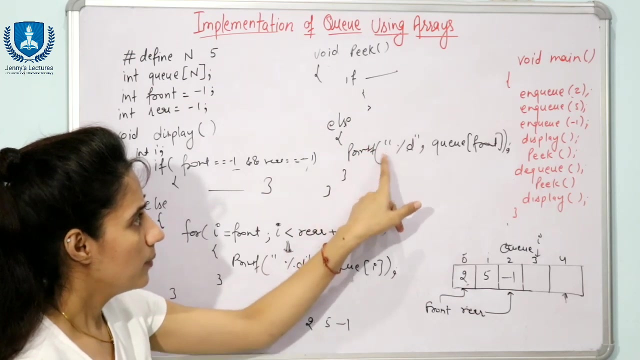 fine the data at the front. so simply you will print here, write printf- %d. you can write the data at front is then %d and here you will write q and front. in subscript you will write front. in this case this condition is not true because q is not empty. suppose i am taking this case else. print f- percentage dq. 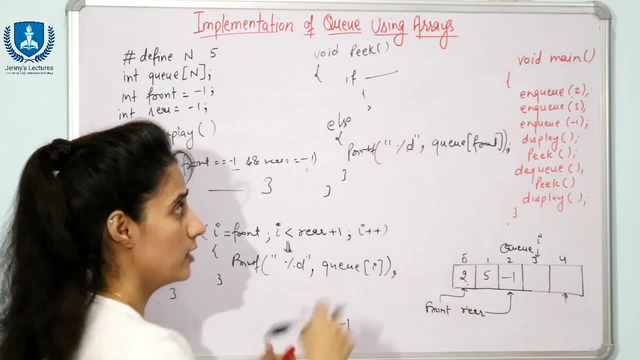 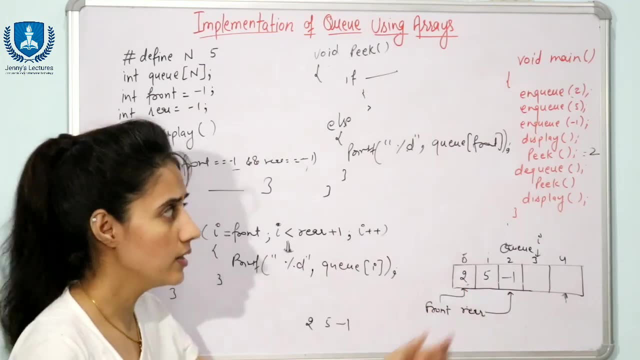 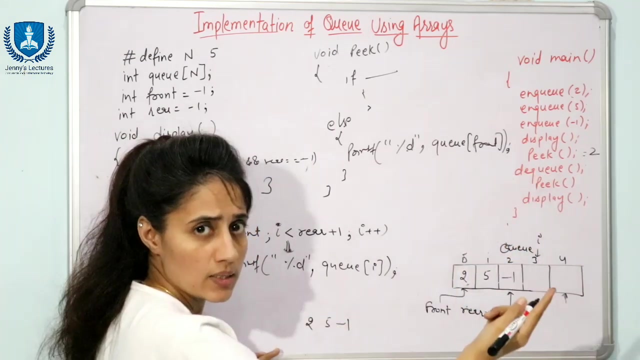 front q is 0 means q of 0 would be printed. that is, 2 would be printed right, and that's it. the front of q is what? 2 only right now and thus display function. would 2, 5 and minus 1. would display 2, 5 minus 1. then dq function. if you will print the data, then it would print 2 after that. 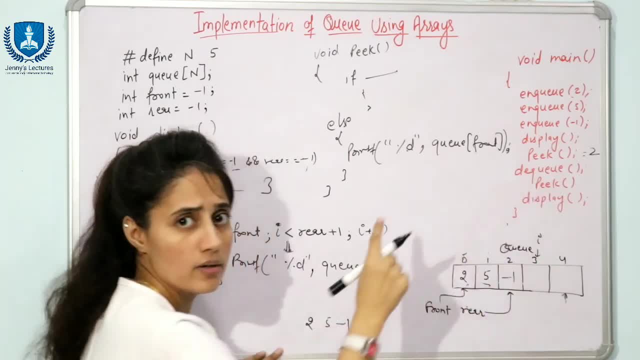 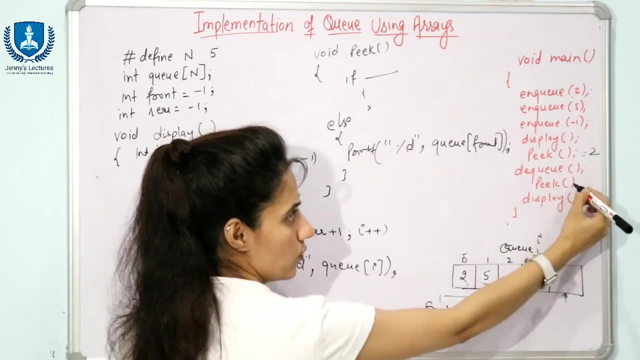 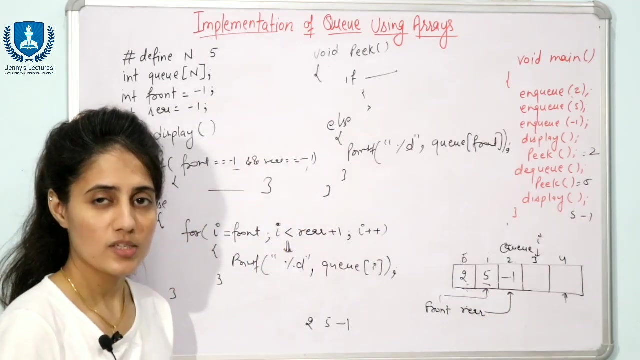 if you will call this peak, then it would print 5, because after 1 dq the front would be pointing to here, front plus, plus, and now q is this one and the front of q is 5. so now this would display 5. display function would display 5 and minus 1: 5 and minus 1. so this is how we can implement a q. 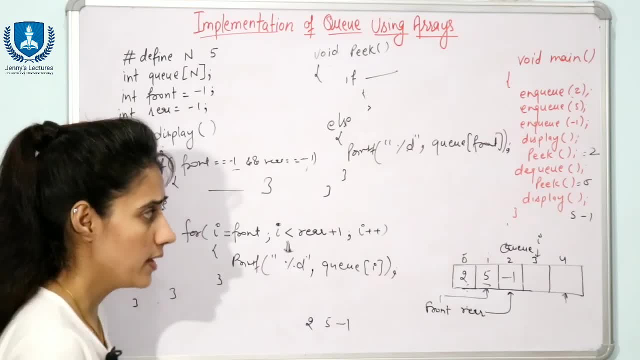 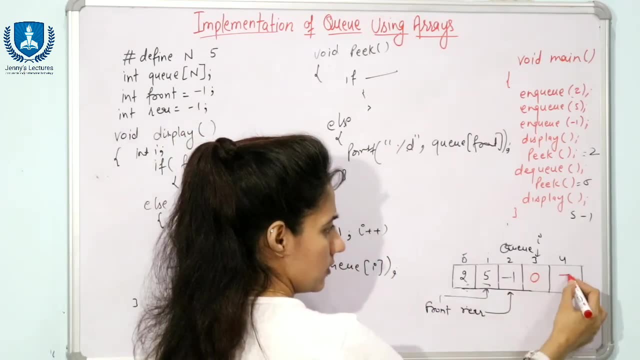 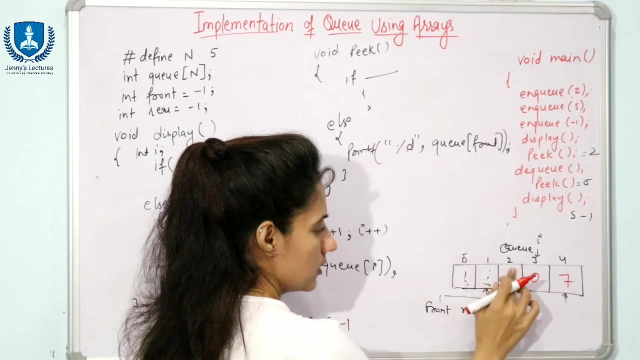 using arrays, right. but here the problem is. the drawback is: suppose the case is i have called nq function 5 times. suppose i have nq'd here 0 and here 7, after that i have dq'd. i have called the dq'd function 3 times: 1, 2 and 3. so this, this, this i have deleted. 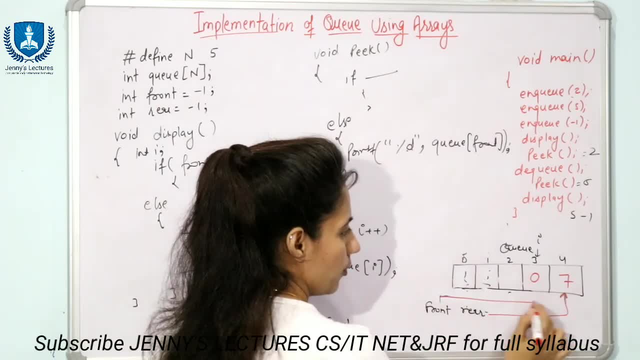 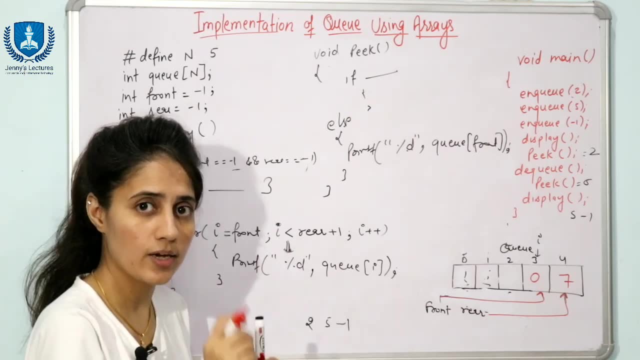 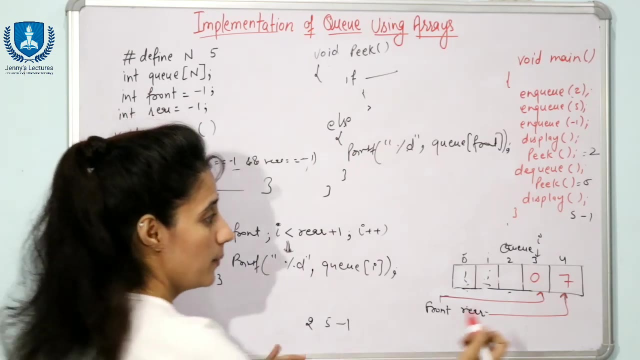 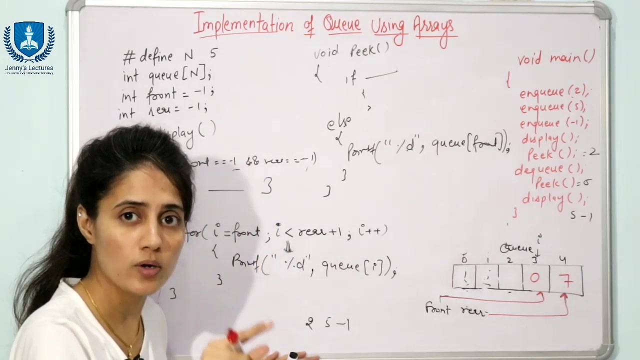 rear would be pointing to here and front would be pointing to here. now suppose this is a q at some point of time. right, and i want to insert some another data. i want i called nq function again. in that case it would show you q is full. why so? because see, condition is what rear is equal to. 4 means rear is maximum size minus 1. 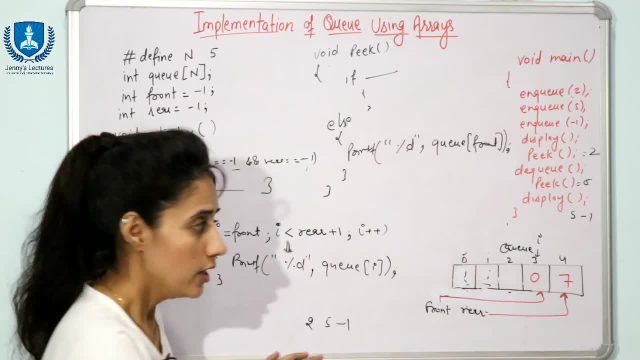 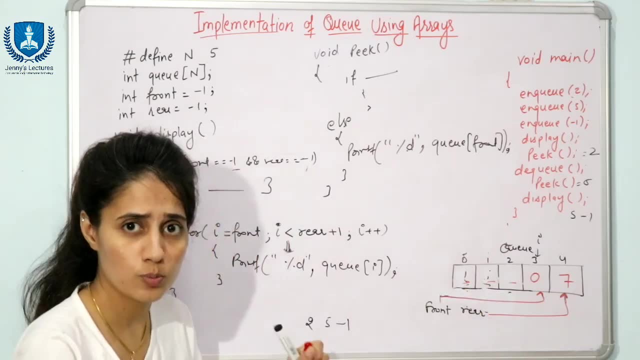 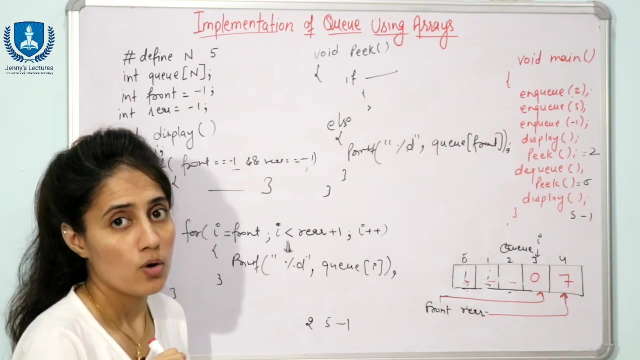 and that we have discussed. that is condition of what q is full. it will show you q is full, but still we have. we have space. now we have three cells left. so this is what wastage of space. space. we cannot insert data here, although we have space, but we cannot insert here now. what if you modify? 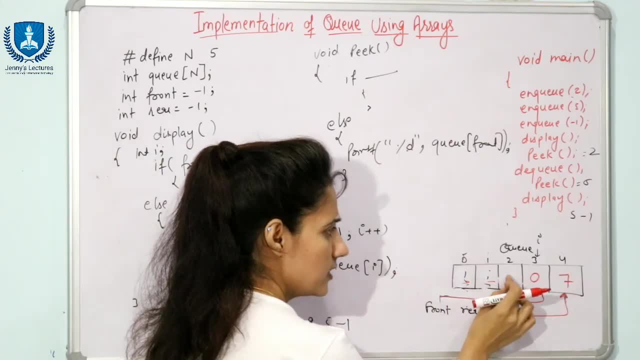 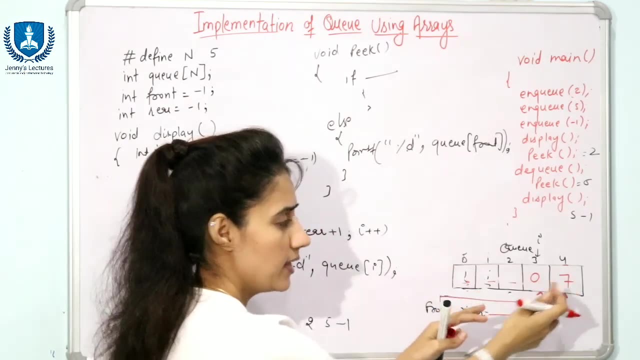 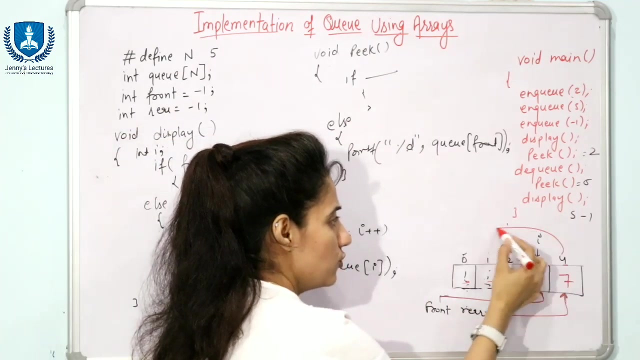 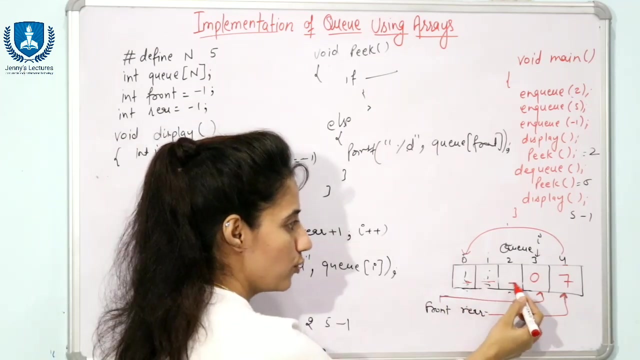 your coding something like that: if there is some space, then what after four? after this four again, if you do some increment in this rear, obviously we will not do rear plus plus, we will modify that thing. so this would give you zero and we can insert here. after that, here also, here also we can insert, right, so this is what a circular. 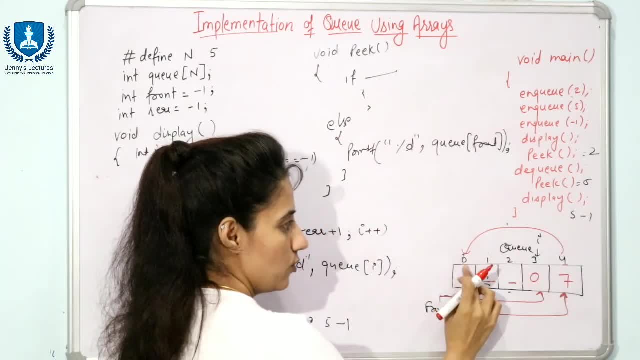 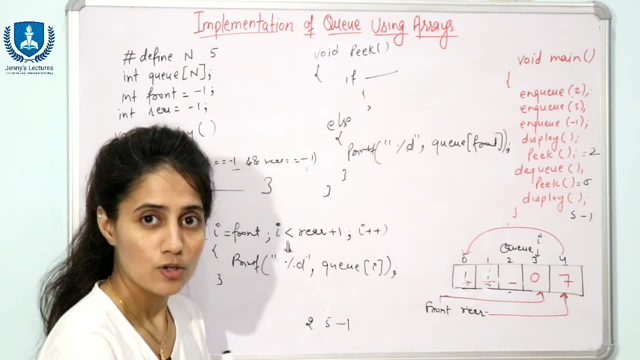 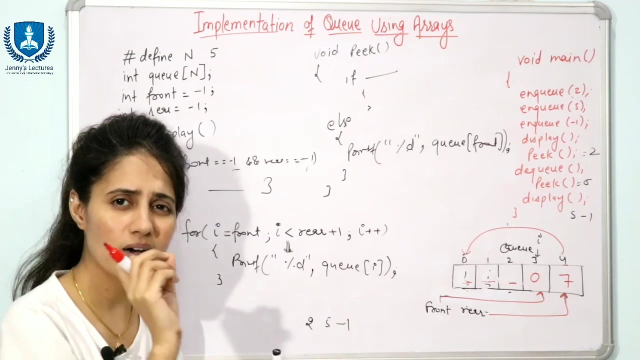 type of thing. right after here again, zero if q is empty, if there is still some space, in that case you can do this thing right. so this is what a circular q? in this case everything would be same. just you have to update a little bit in your nq function and dq function. you cannot simply do front plus, plus in dq and rear plus. 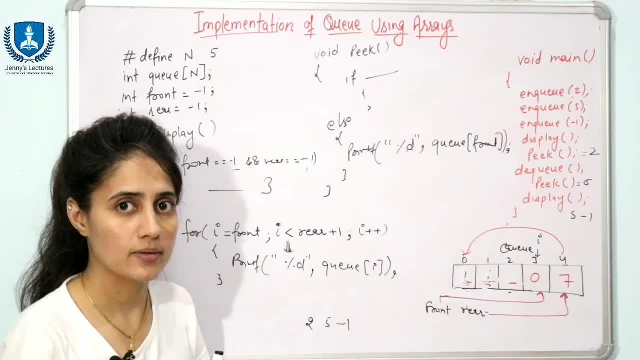 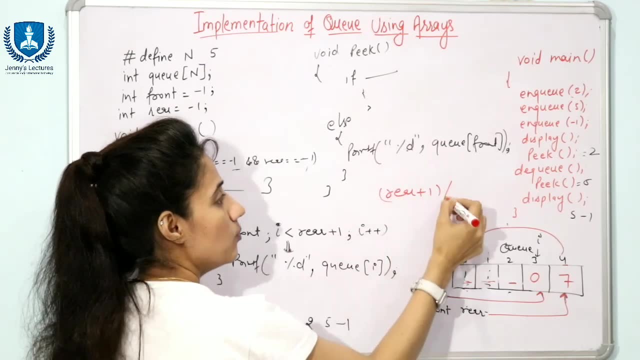 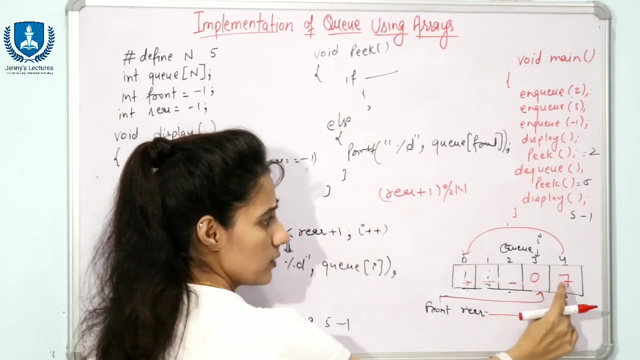 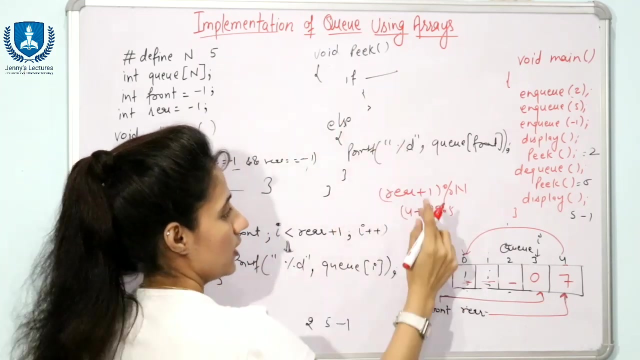 plus in nq- you have to modify that thing a little bit, right- rather than rear plus plus, what you will do. this one is rear plus one and n is zero. so here, this one is here, and one sale is four, right. so how do we know? theâu value of the private is zero, it is 4right, it is n and n is 0, right. so what? welcome?